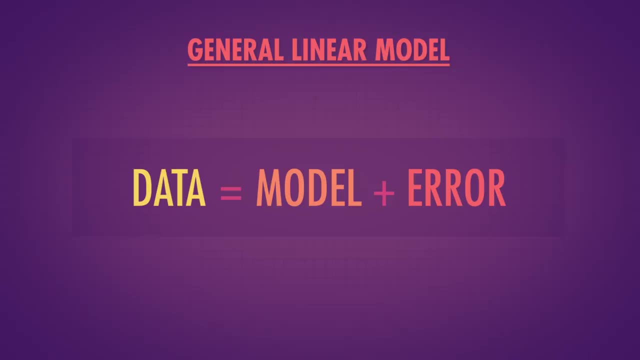 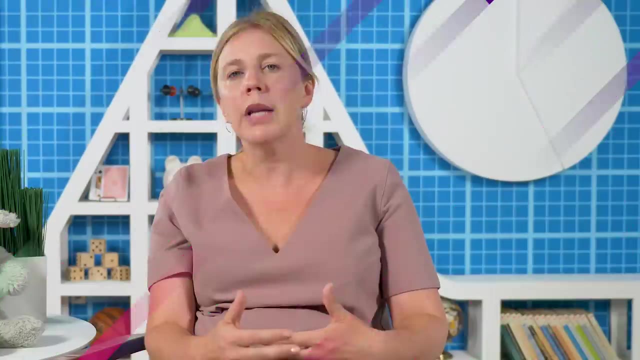 two piles Information that can be explained by a model that represents the way we think things work and error, which is the amount of information that our model fails to explain. So let's apply that to a new model, the ANOVA. 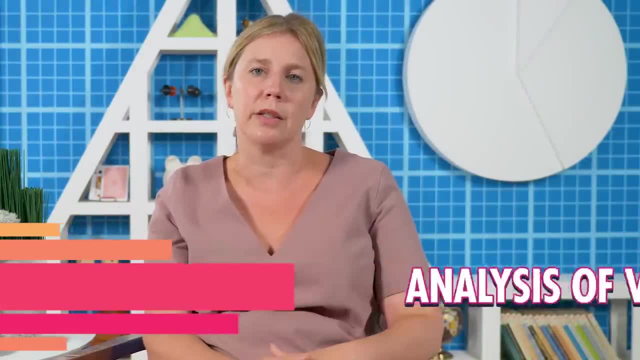 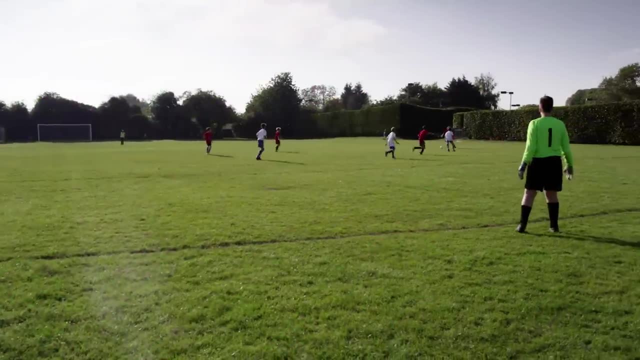 ANOVA is an acronym for Analysis of Variance. It's actually really similar to regression, except we're using a categorical variable to predict a continuous one, Like using a soccer player's position to predict the number of yards he runs in a game. 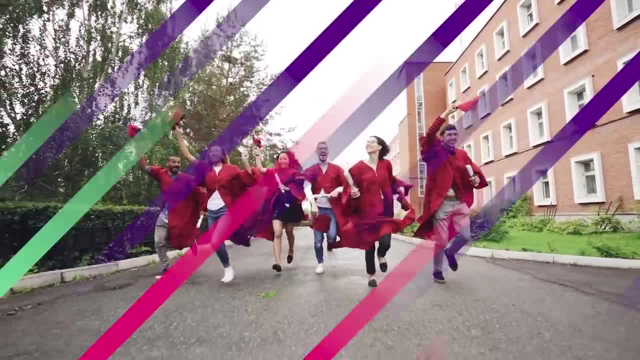 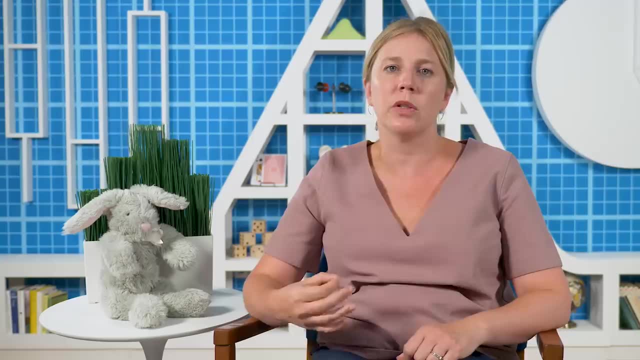 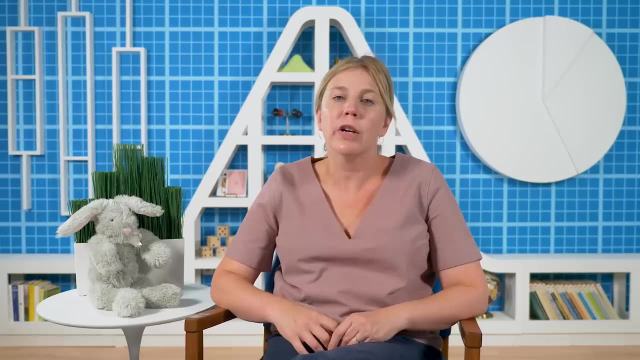 Or using highest completed degree to predict a person's salary, And note here that this alone isn't evidence that getting a degree causes a higher salary, Just that knowing someone's degree might help estimate how much they get paid. Like regression, the ANOVA builds a model of how the world works. 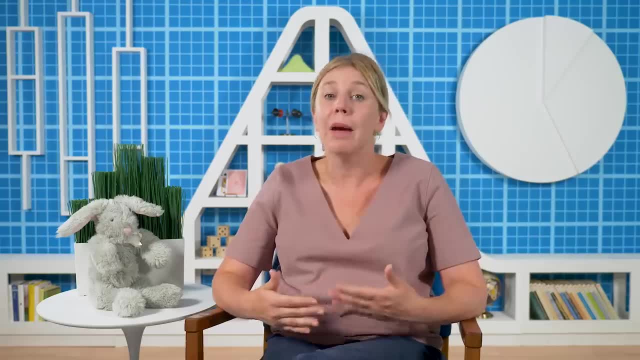 For example, my model of how many bunnies I'll see on my walk into work might be that if it's raining I'll see one bunny, And if it's sunny I'll see five. I walk through a bunny preserve. 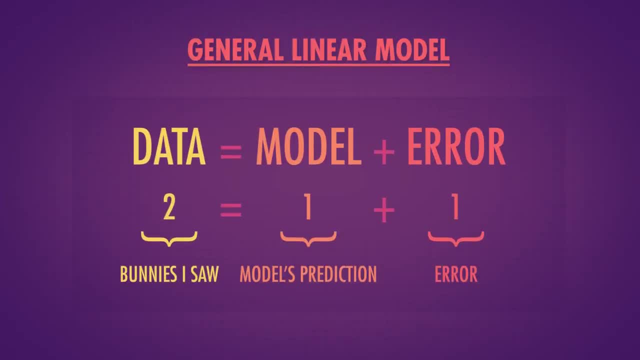 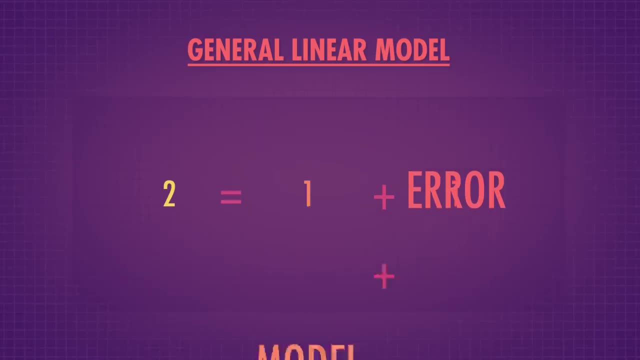 One and five are my predictions for how many bunnies I'll see, based on whether or not it's raining. Yesterday it rained And I saw two bunnies. My model predicted one And my error is one, And we can represent this model as a sort of regression where there are only two possible. 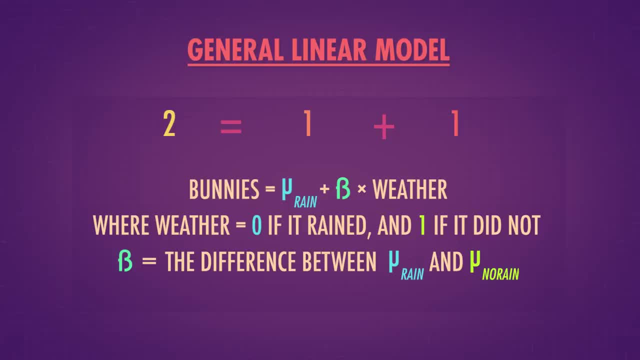 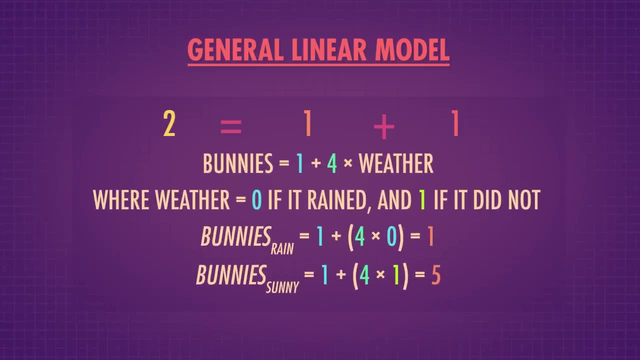 values that the variable weather can have: Zero if it rains or one if it doesn't. In this case, expected number of bunnies on a rainy day is one And beta is the difference between the two means Five minus one is four. 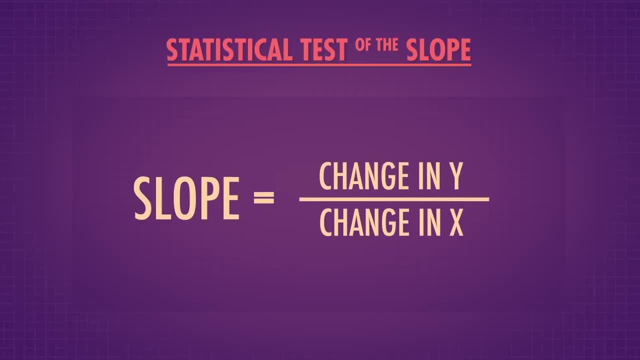 Which means our ANOVA model looks like this: In a regression, we did a statistical test of the slope, And that's what the simple ANOVA is doing too. Since we assigned rainy days to be coded as zero and sunny days as one, the change in 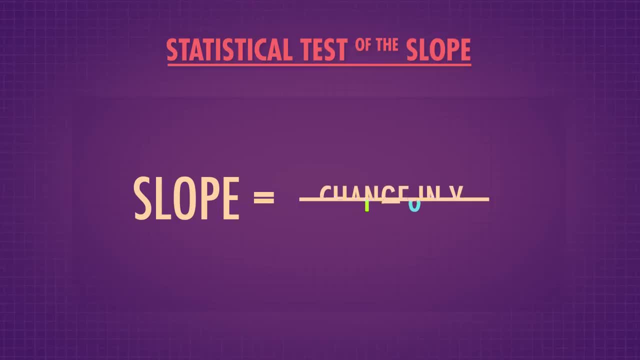 the X direction is just one, One minus zero. So the slope of this line is the difference between mean bunny counts on sunny days, five minus mean bunny counts on rainy days, one. The difference of four is the change in the Y direction. 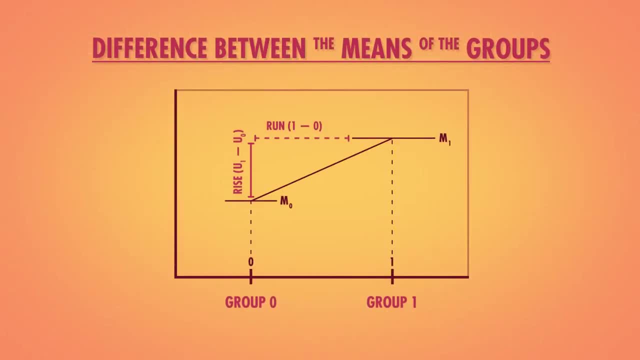 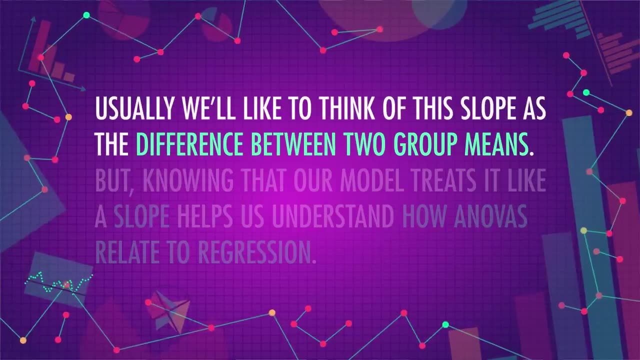 We test this difference in the same way we tested the regression slope, And the slope tells us the difference between the means of the two groups. Usually, we'll like to think of this slope as the difference between two group means, But knowing that our model treats it like a slope helps us understand how ANOVAs relate. 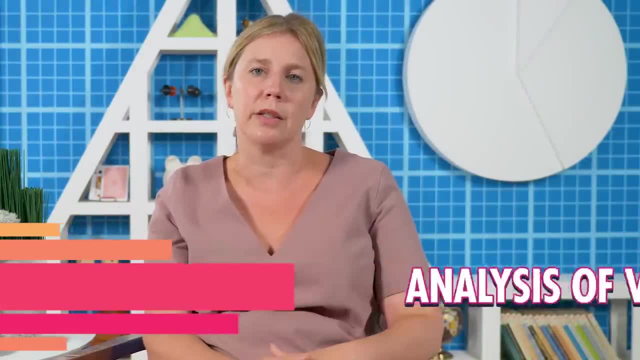 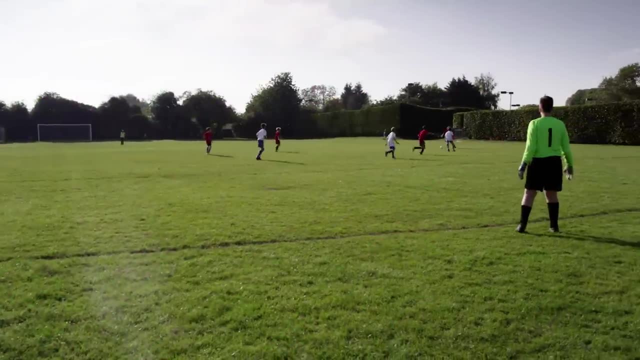 ANOVA is an acronym for Analysis of Variance. It's actually really similar to regression, except we're using a categorical variable to predict a continuous one, Like using a soccer player's position to predict the number of yards he runs in a game. 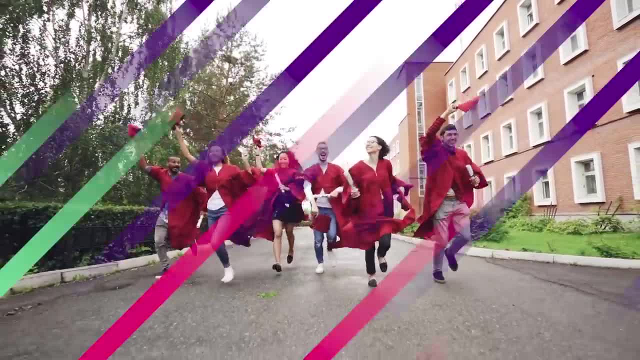 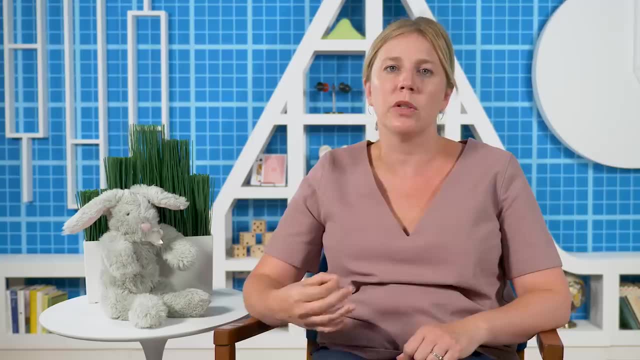 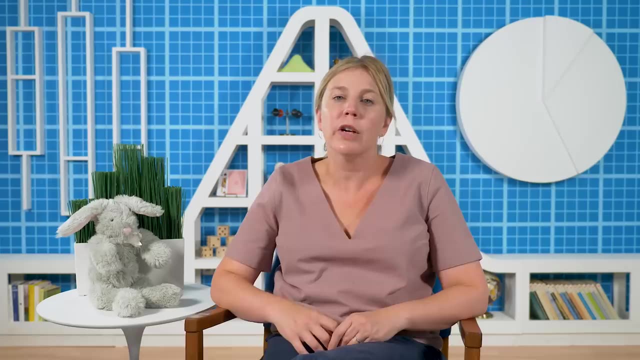 Or using highest completed degree to predict a person's salary, And note here that this alone isn't evidence that getting a degree causes a higher salary. just that knowing someone's degree might help estimate how much they get paid. Like regression, the ANOVA builds a model of how the world works. 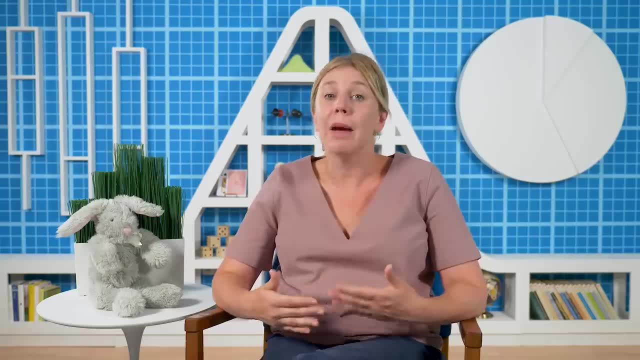 For example, my model of how many bunnies I'll see on my walk into work might be that if it's raining I'll see one bunny and if it's sunny I'll see five. I walk through a bunny preserve. 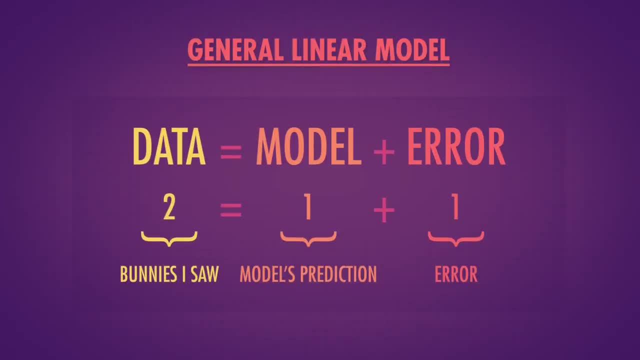 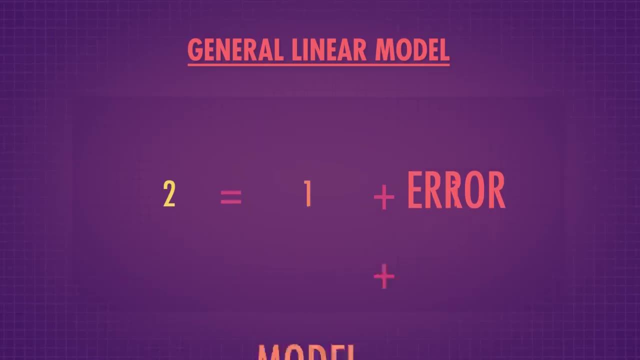 One and five are my predictions for how many bunnies I'll see, based on whether or not it's raining. Yesterday it rained And I saw two bunnies. My model predicted one and my error is one, And we can represent this model as a sort of regression where there are only two possible. 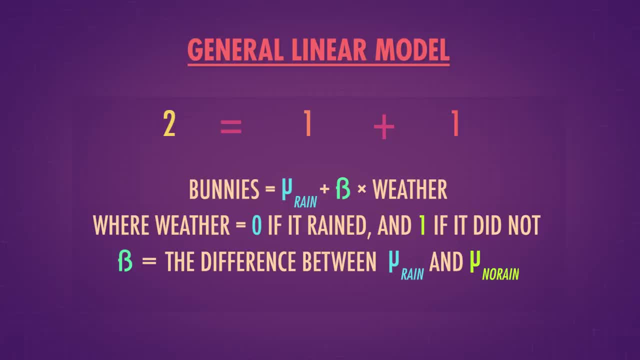 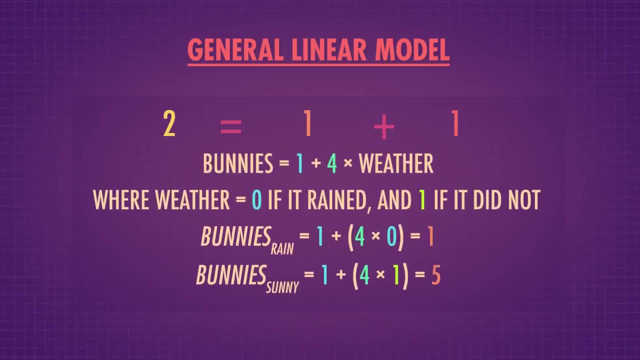 values that the variable weather can have: Zero if it rains or one if it doesn't. In this case, expected number of bunnies on a rainy day is one And beta is the difference between the two means Five minus one is four. 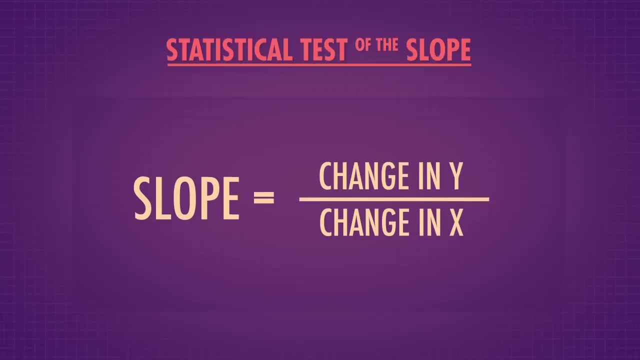 Which means our ANOVA model looks like this: In a regression we did a statistical test of the slope. ANOVA is doing two, Since we assigned rainy days to be coded as zero and sunny days as one. the change in 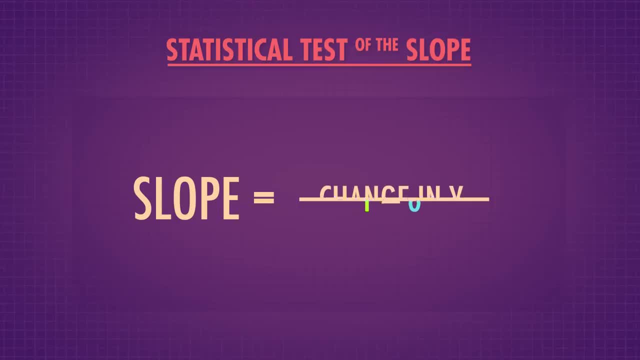 the X direction is just one, One minus zero. So the slope of this line is the difference between mean bunny counts on sunny days, five minus mean bunny counts on rainy days, one. The difference of four is the change in the Y direction. 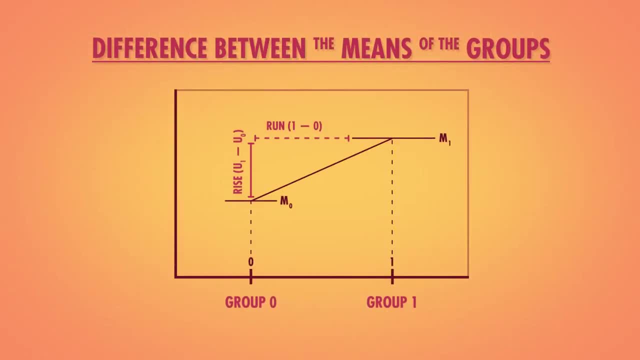 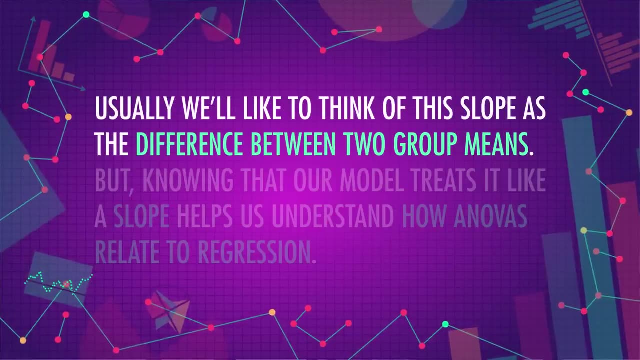 We test this difference in the same way we tested the regression slope, And the slope tells us the difference between the means of the two groups. Usually, we'll like to think of this slope as a mean. A slope is a difference between two group means. 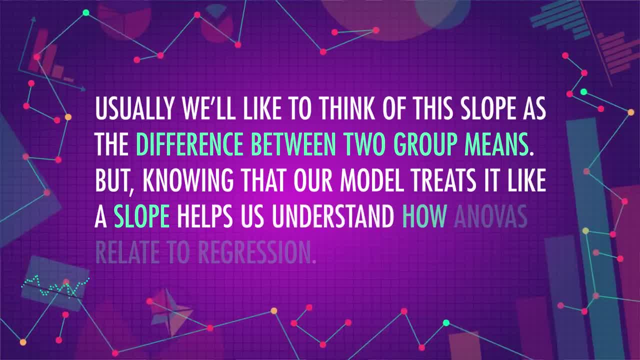 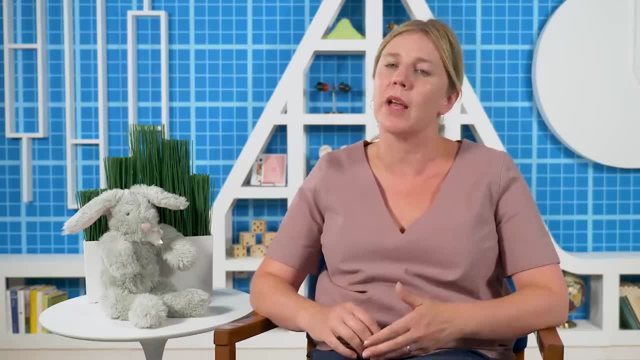 But knowing that our model treats it like a slope helps us understand how ANOVAs relate to regression. In a regression, the slope tells you how much an increase in one unit of X affects Y, Like, for example, how much an increase of one year increases shoe size in kids. 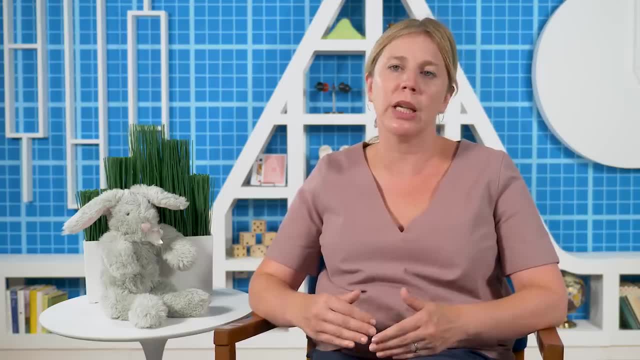 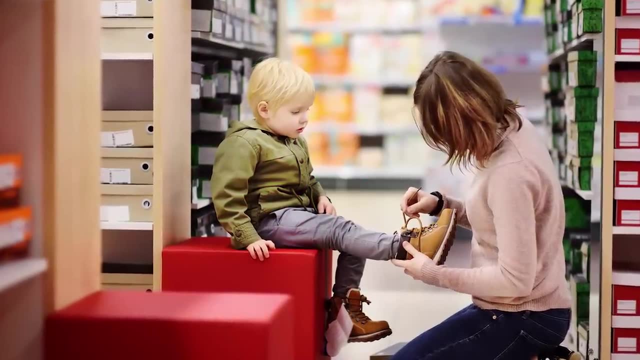 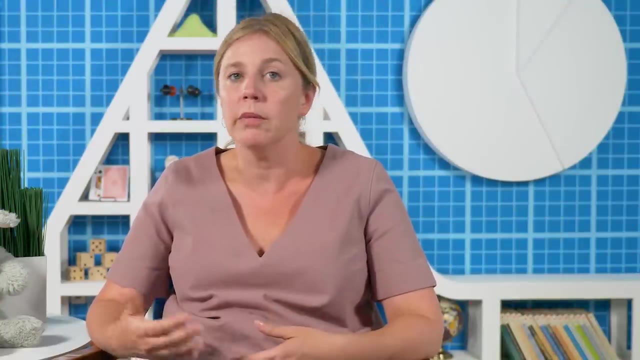 to regression. In a regression, the slope tells you how much an increase in one unit of X affects Y, Like, for example, how much an increase of one year increases shoe size in kids. An ANOVA actually does the same thing. It looks at how much an increase from zero to one affects the number. 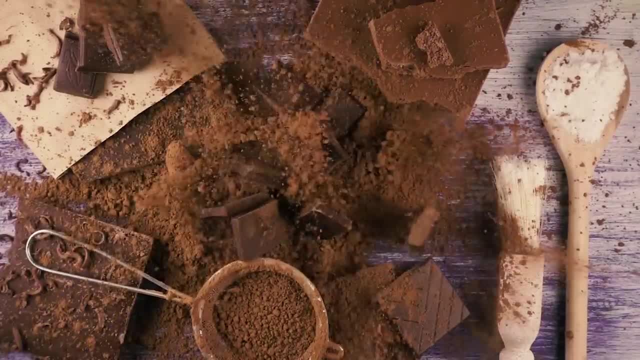 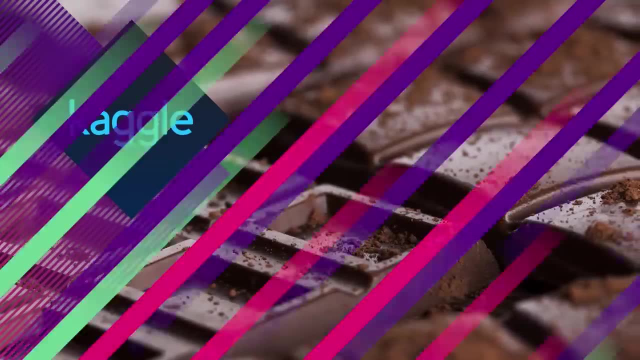 of bunnies you'd see. Now to another example. let's look at the ratings of various chocolate bars based on the type of cocoa bean used. We'll use a dataset you can find at Kagglecom, courtesy of Brady Berlinski. 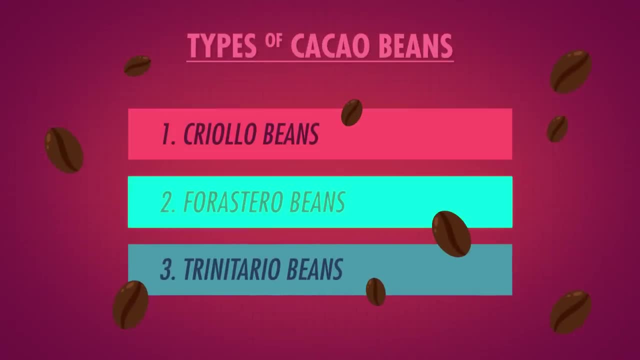 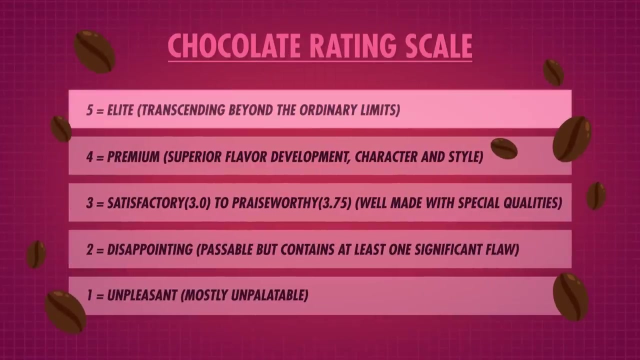 Our three groups are chocolate bars made with Criollo beans, Forastero beans or Trinitario beans. Chocolate making is complex, so we took a small sample of bars that only contained one of these three beans, And the chocolate taster used a scale with five as the highest score, transcending beyond 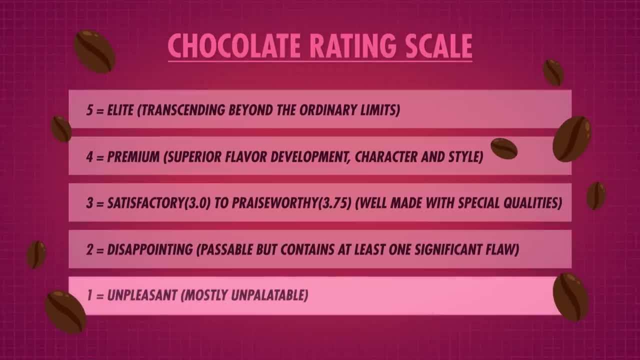 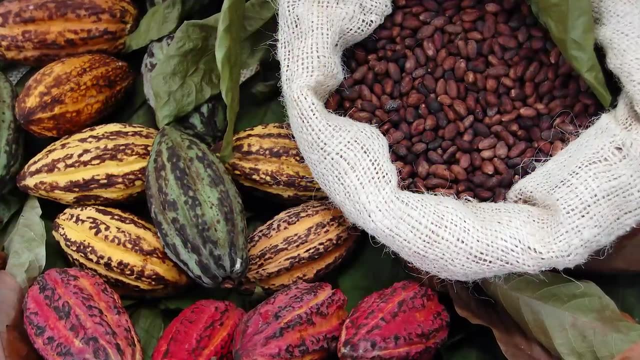 the ordinary limits. One was mostly unpalatable, But is there really mostly unpalatable chocolate out there? We want to know if the type of beans affects our taster's ratings. To find out, we need the ANOVA model. 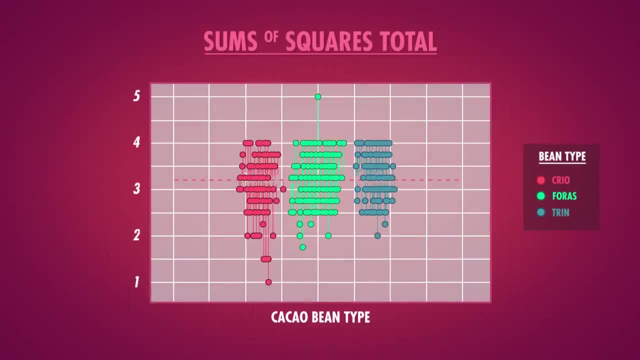 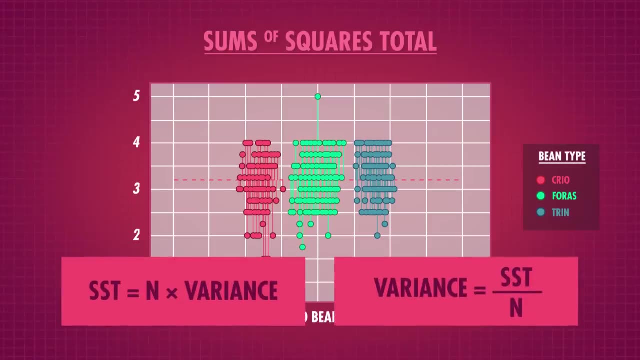 Like regression, we can calculate the sums of squares total by adding up the squared differences between each chocolate rating and the overall mean chocolate rating. This gives us our sums of squares total, or SST. If that sounds like how we calculated variance, that's because it is. 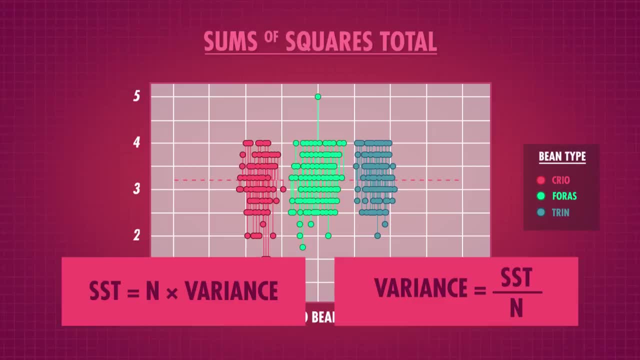 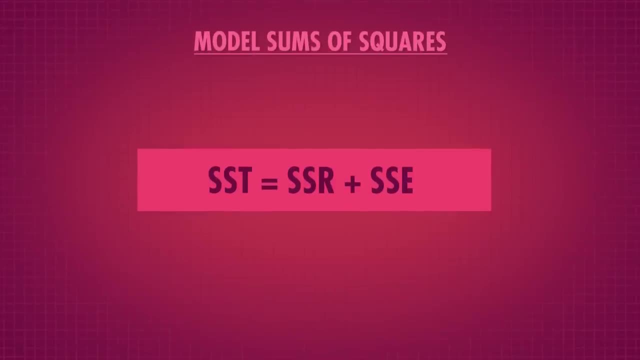 SST is just n times variance. The sum represents the total amount of variation or information in the data. Now we need to partition this variation. When we previously used a simple linear regression model, we partitioned this variation into two parts: Sums of squares for regression and sums of squares for error. 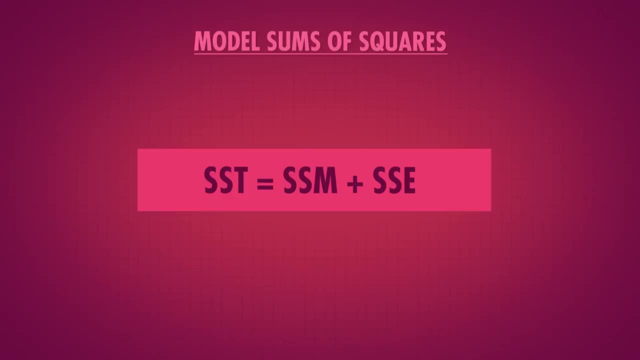 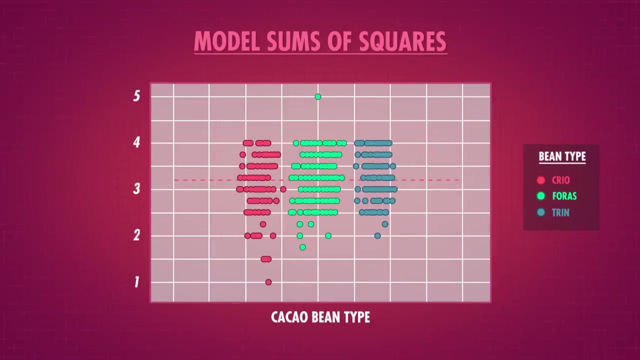 And the ANOVA does the same thing. The first step is to figure out how much of the variation is explained by our model In an ANOVA, what we're using here. our best guess of a chocolate bar's rating is its group mean. 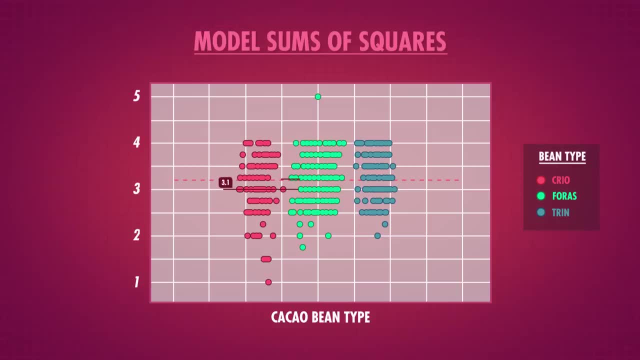 For bars made with Criollo beans 3.1,, Forastero beans 3.25, and Trinitario beans 3.27.. So we sum up the squared distances between each point and its group mean. This is called our model, sums of squares or SSM, because it's the variation, our model. 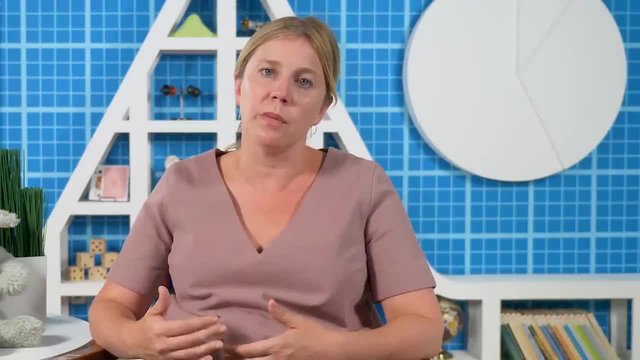 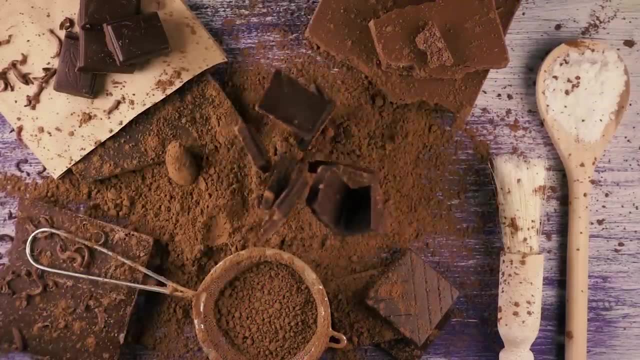 An ANOVA actually does the same thing. It looks at how much an increase from zero to one affects the number of bunnies you'd see. Now to another example. Let's look at the ratings of various chocolate bars based on the type of cocoa bean used. 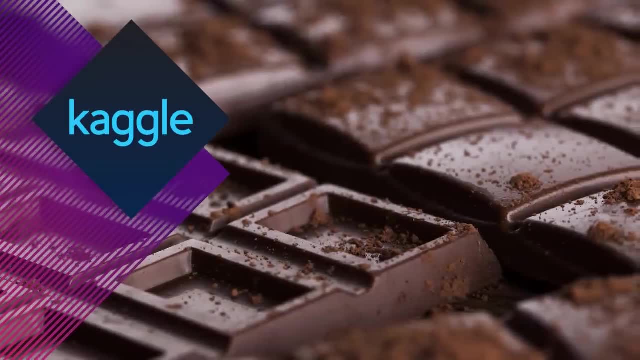 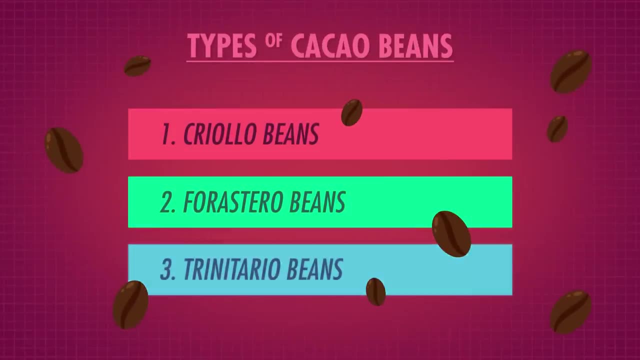 We'll use a dataset you can find at Kagglecom, courtesy of Brady Berlinski. Our three groups are chocolate bars made with Criollo beans, Forastero beans or Trinitario beans. Chocolate making is complex, so we took a small sample of bars that only contained one. 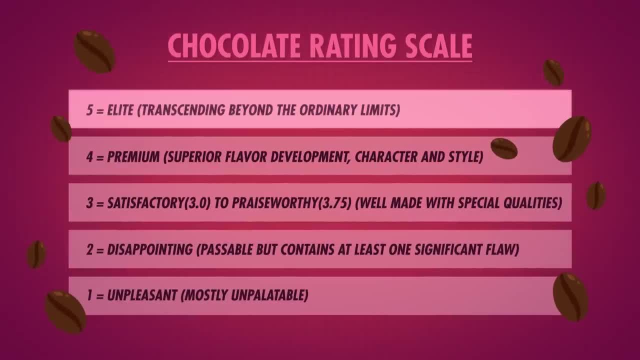 of these three beans And the chocolate taster used a scale with five as the highest score, transcending beyond the ordinary limits. One was mostly chocolate, The other was mostly unpalatable. But is there really mostly unpalatable chocolate out there? 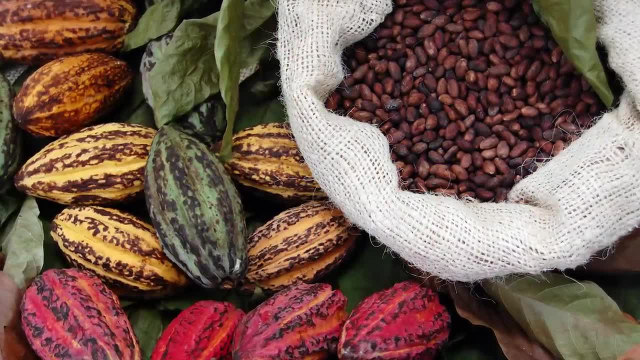 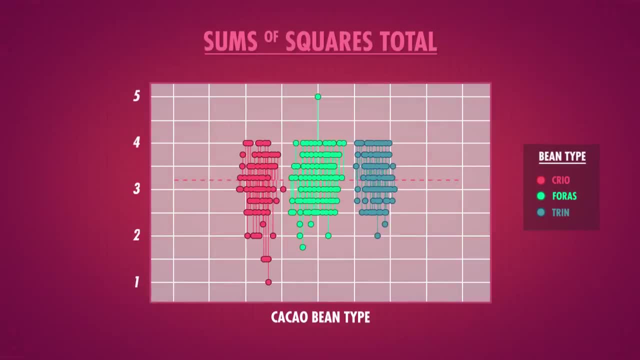 We want to know if the type of beans affects our taster's ratings. To find out we need the ANOVA model. Like regression, we can calculate the sums of squares total by adding up the squared differences between each chocolate rating and the overall mean chocolate rating. 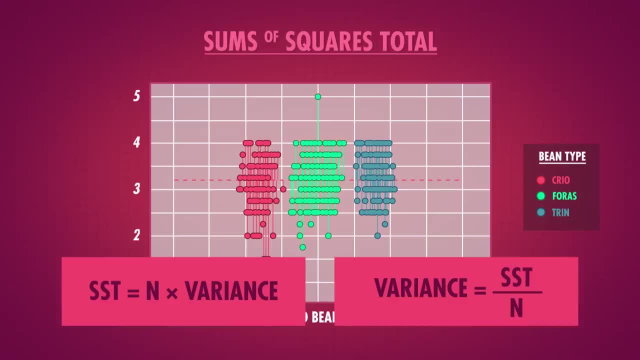 This gives us our sums of squares: total or SST. If that sounds like how we calculated variance, that's because it is SST is just n times variance. The sum represents the total amount of variation or information in the data. Now we need to partition this variation. 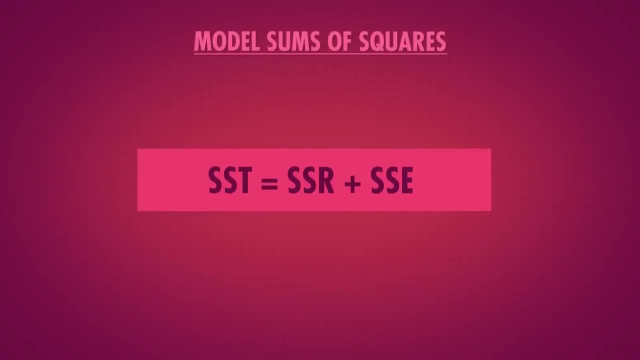 When we previously used a simple linear regression model, we partitioned this variation into two parts- Sums of squares for regression and sums of squares for error, And the ANOVA does the same thing. The first step is to figure out how much of the variation is explained by our model. 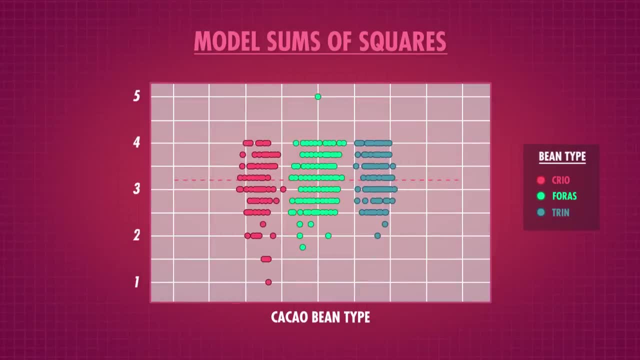 In an ANOVA, what we're using here, our best guess of a chocolate bar's rating is its group mean. In the ANOVA model, the number of chocolate bars is equal to the number of chocolate bars. The number is made with CREOLO beans 3.1,, FORESTERO beans 3.25, and TRINITARIO beans. 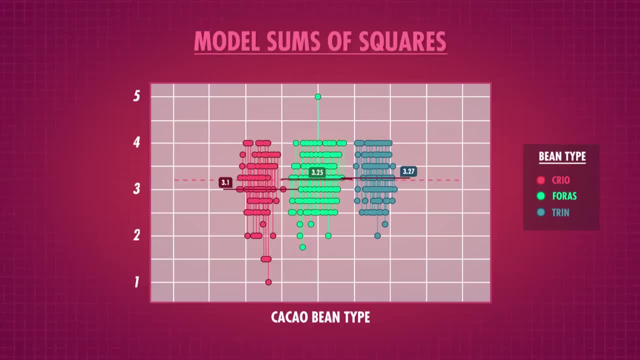 3.27.. So we sum up the squared distances between each point and its group mean. This is called our model sums of squares or SSM, because it's the variation our model explains. So now we have the amount of variation explained by the model. 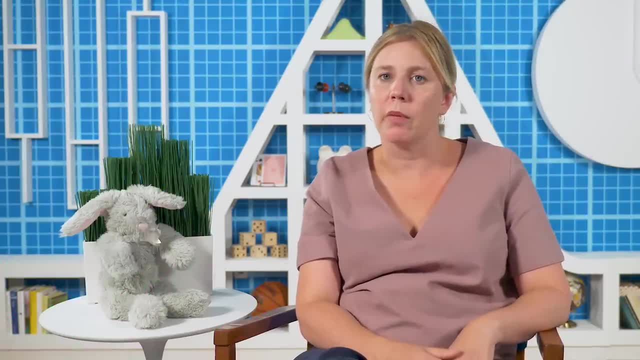 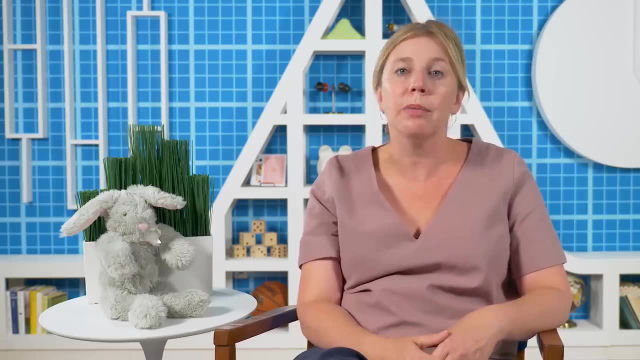 explains. So now we have the amount of variation explained by the model, In other words, how much variation is accounted for. if we just assumed each rating value were its group mean rating, We're also going to need the amount of variation that it doesn't explain. 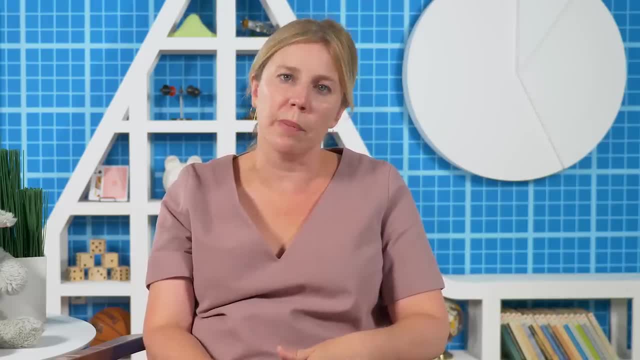 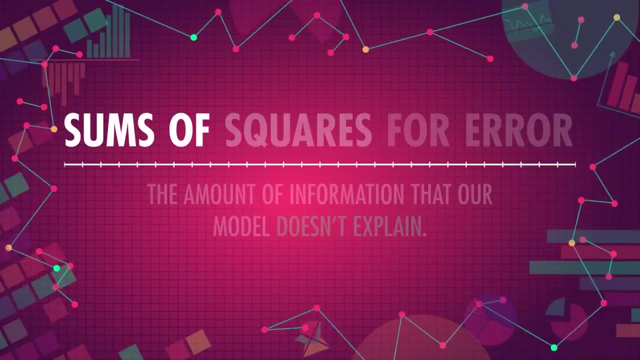 In other words, how much ratings vary within each group of cocoa beans. So we can sum up: the squared differences between each data point and its group mean to get our sums of squares for error, The amount of information that our model doesn't explain. 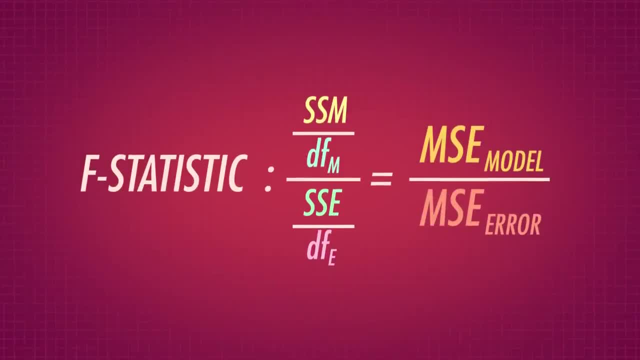 Now that we have that information, we can calculate our F-statistic just like we did for regression. The F-statistic compares how much variation our model accounts for Versus how much it can't account for. The larger that F is, the more information our model is able to give us about our chocolate. 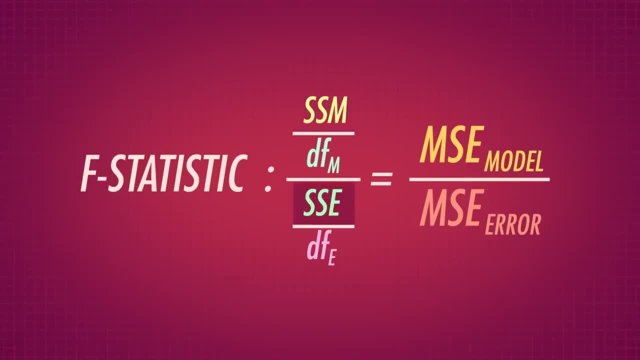 bar ratings. Again, SSM is the variation our model explains and SSE is the variation it doesn't explain. We want to compare the two, but we also need to account for the amount of independent information that each one uses. So we divide each sums of squares by its degrees of freedom. 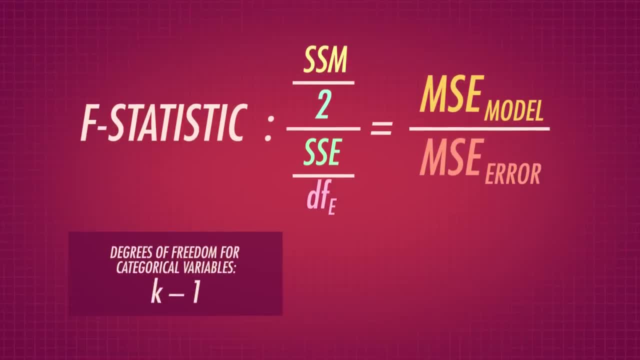 Our ANOVA model has two degrees of freedom. In general, the formula for degrees of freedom for categorical variables Like cocoa bean types And an ANOVA is k-1, where k is the number of groups. In our case, we have three groups. 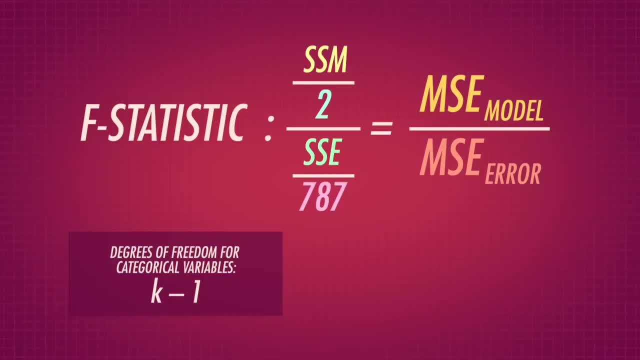 Our sums of squares for error has 787 degrees of freedom Because we originally had 790 data points but we calculated three means. The general formula for degrees of freedom for your errors is n-k, where n is the sample size and k is the number of groups. 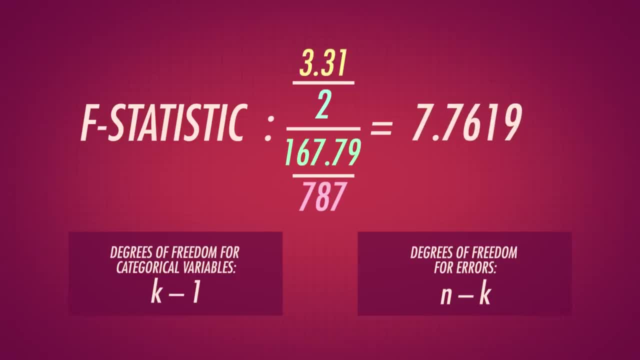 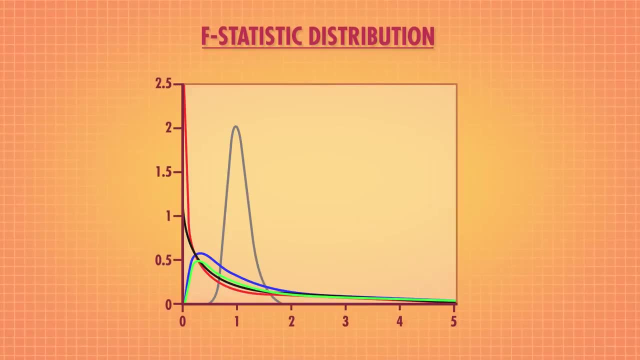 For our test, we got an F-statistic of 7.7619.. This F-statistic is the number of groups. The F-statistic, sometimes called an F-ratio, has a distribution that looks like this, And we're going to use this distribution to find our p-value. 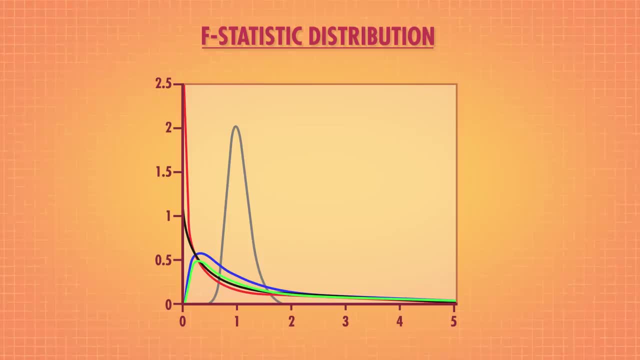 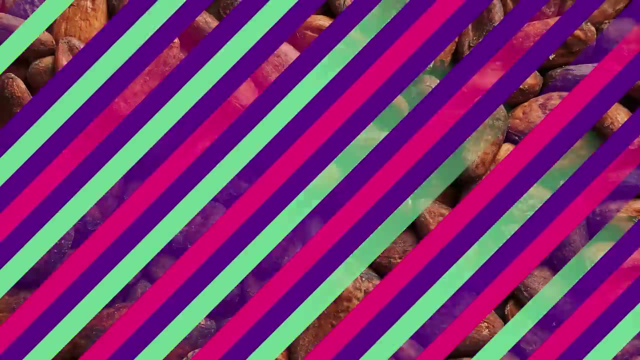 We want to know whether the effect of bean type on chocolate bar ratings is significant. In this case we have a p-value of 0.000459, small enough to reject the null, So we found evidence that beans influence the chocolate bar ratings. 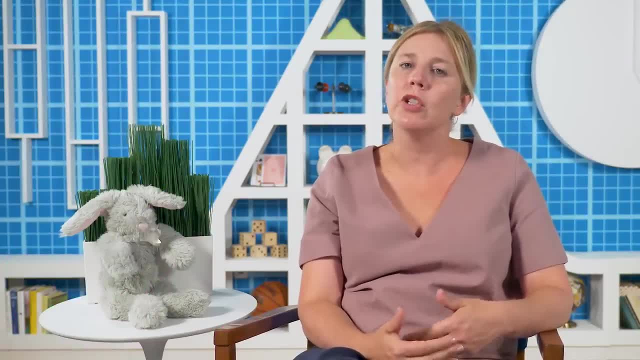 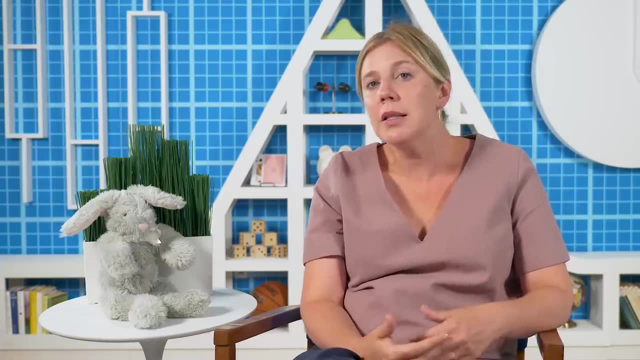 In other words, how much variation is accounted for. if we just assumed each rating value were its group mean, We're also going to need the amount of variation that it doesn't explain, In other words, how much ratings vary within each group of cocoa beans. 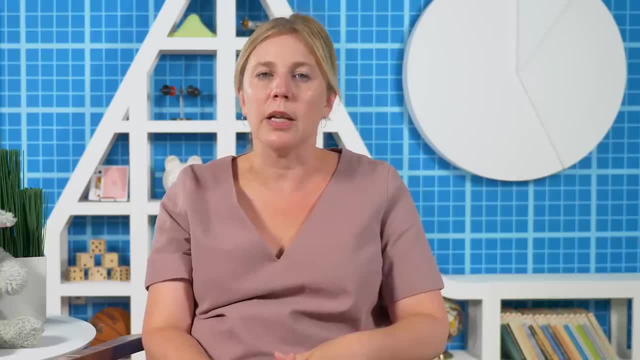 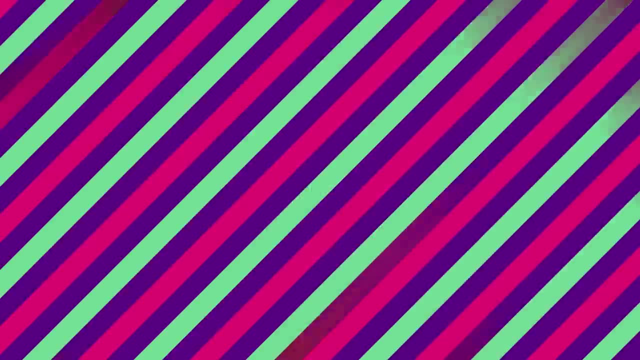 So we can sum up the squared differences between each data point and its group, mean to get our sums of squares for error, the amount of information that our model doesn't explain. Now that we have that information, we can calculate our F-statistic just like we did. 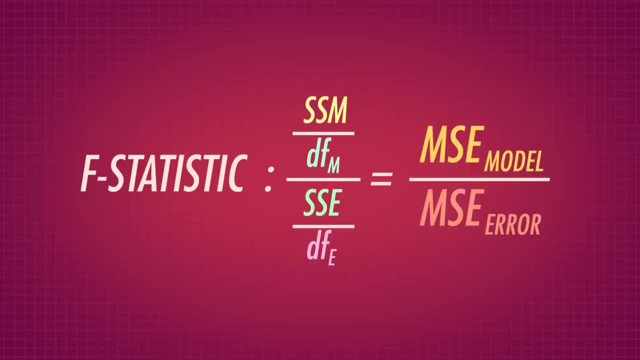 for regression. The F-statistic compares how much variation our model accounts for Versus how much it can't account for. The larger that F is, the more information our model is able to give us about our chocolate bar ratings. Again, SSM is the variation our model explains and SSE is the variation it doesn't explain. 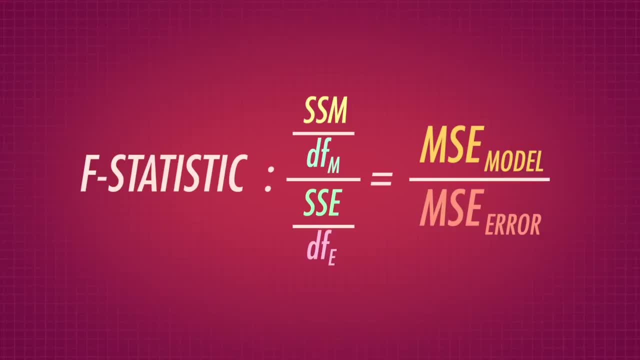 We want to compare the two, but we also need to account for the amount of independent information that each one uses. So we divide each sums of squares by its degrees of freedom. Our ANOVA model has two degrees of freedom In general. the formula for degrees of freedom for categorical variables like cocoa bean. 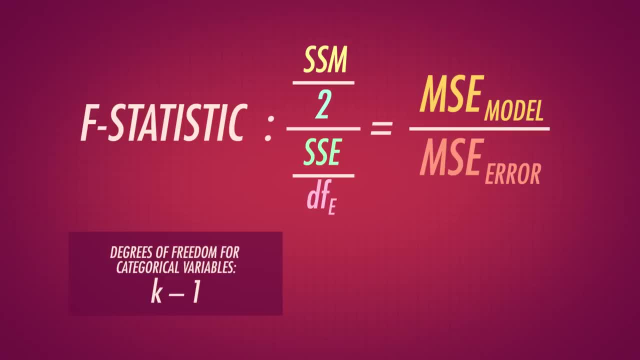 types in an ANOVA is k-1, where k is the number of groups. In our case we have three groups. Our sums of squares for error has 787 degrees of freedom, because we originally had 790 data points but we calculated three means. 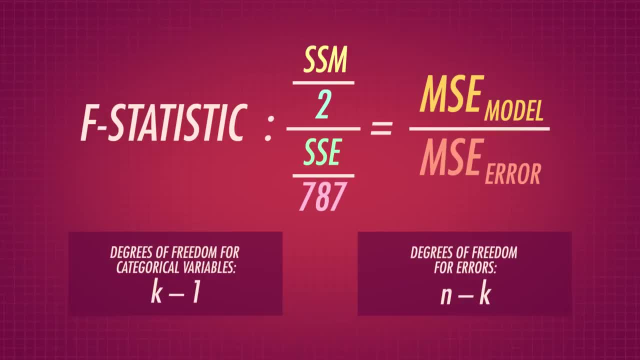 The general formula for degrees of freedom for your errors is n-k, where n is the sample size and k is the number of groups. For our test, we got an F-statistic of 7.7619.. This F-statistic, sometimes called the F-statistic, can be used to calculate the number of groups. 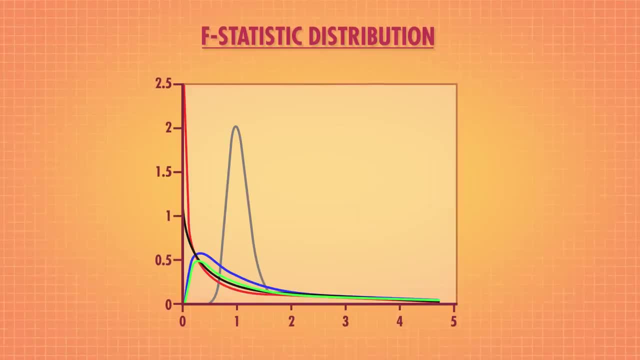 For our test, we got an F-statistic of 7.7619.. For our test, we got an F-statistic of 7.7619.. For our test, we got an F-statistic, sometimes called the F-ratio has a distribution that: 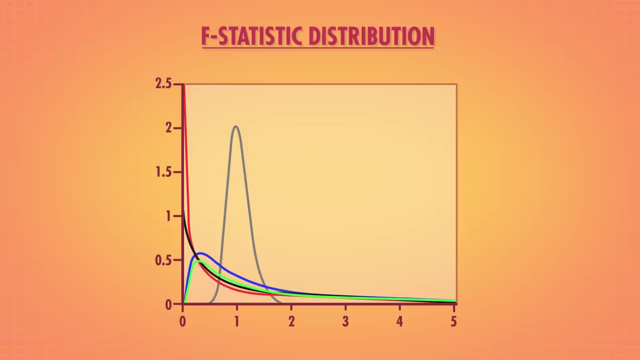 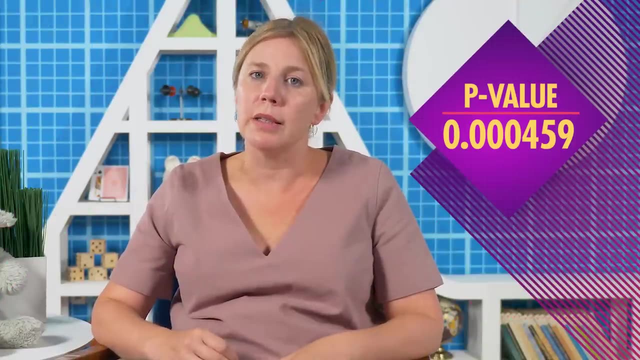 looks like this, And we're going to use this distribution to find our p-value. We want to know whether the effect of bean type on chocolate bar ratings is significant. In this case, we have a p-value of 0.000459, small enough to reject the null. 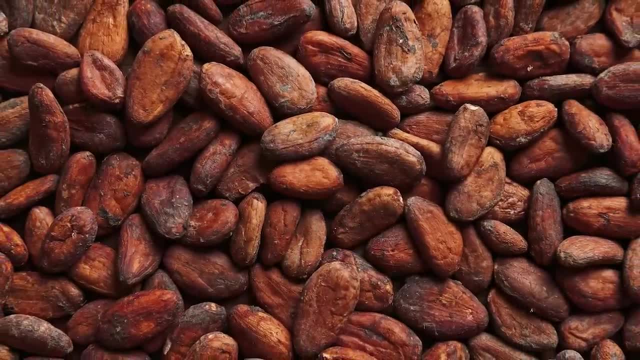 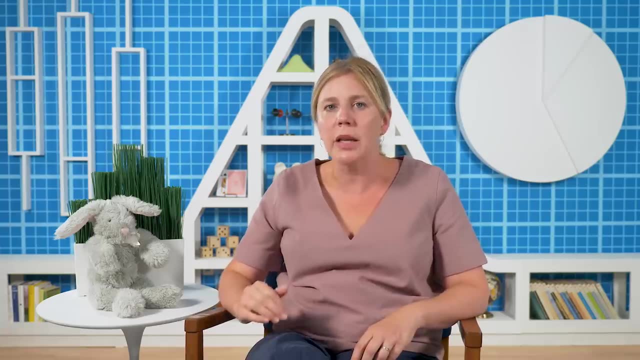 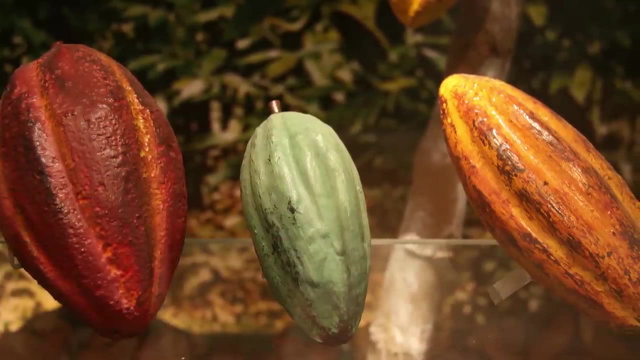 So we found evidence that beans influence the chocolate bar ratings. A statistically significant result means that there's some statistically significant difference somewhere in the groups, but it doesn't tell us where that difference is. Maybe Trinitario is significantly different from Criollo, but not for Astero beans. 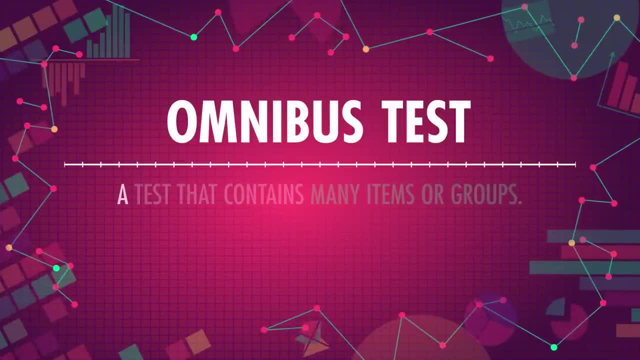 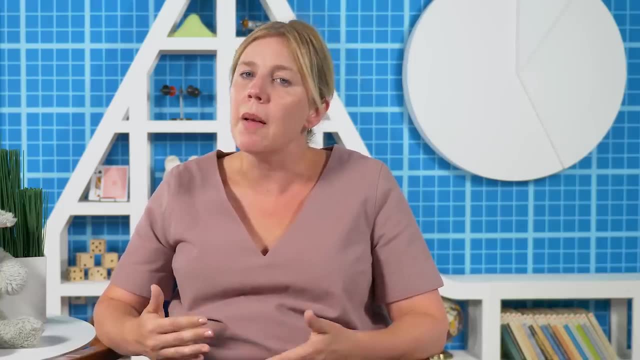 An F-test is an example of an omnibus test, which means it's a test that contains many items or groups. When we get a significant F-statistic, it means that there's some statistically significant difference somewhere between the groups, but we still have to look for it. 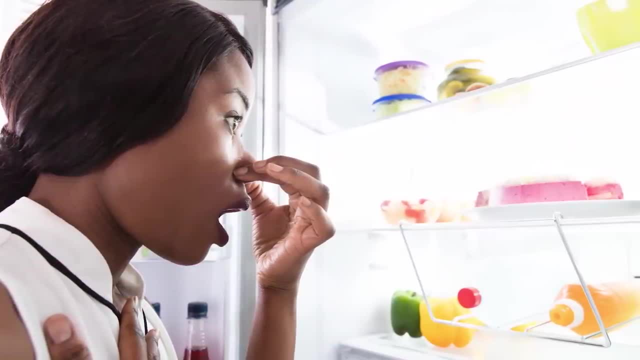 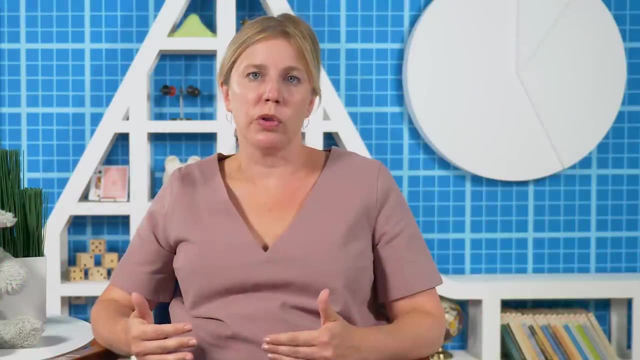 It's kind of like walking into your kitchen and smelling something really stinky. You know there's something gross, but you have to do more work to find out exactly what's rotting. We already have tools to do this, in statistics at least, because you can follow up. 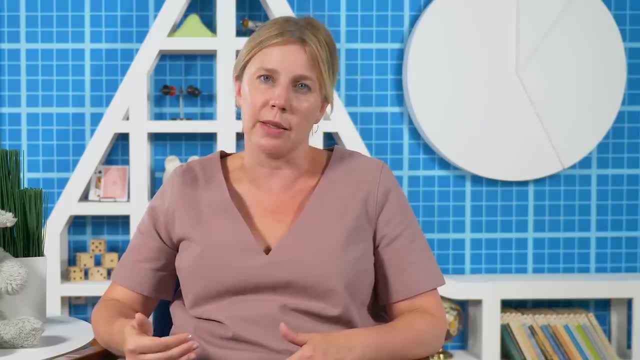 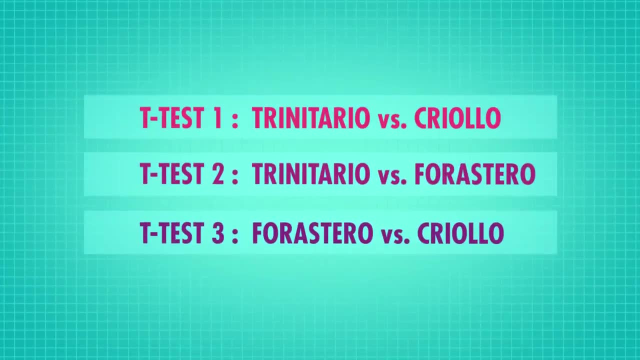 a significant F-test in an ANOVA with multiple t-tests, one for every unique pair of categories your variable had, We had three, which means we only need to do three t-tests in order to find the statistically significant difference or differences. To conduct these t-tests, we just 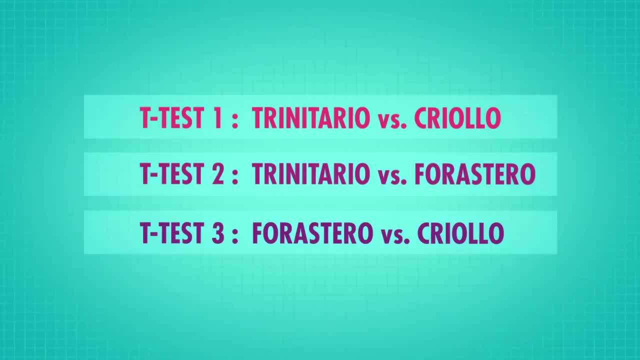 take the data in the two categories for that t-test and calculate the t-statistic and p-value. For our first t-test we just look at the bars with Trinitario and Criollo beans First. we follow our test statistic general formula. We take the difference between the 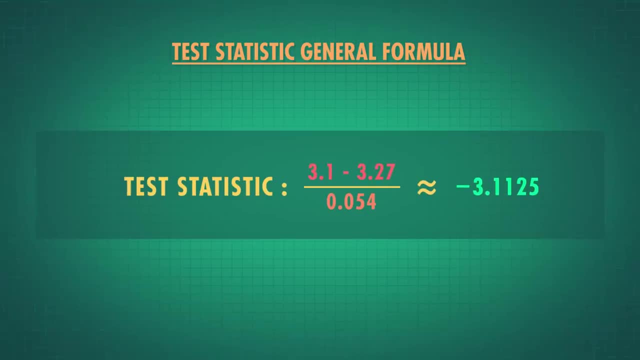 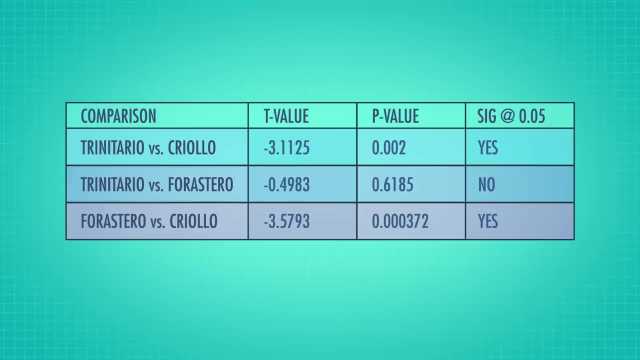 mean rating of chocolates made with Trinitario and Criollo beans and divide by the standard error, And once we do this for all three comparisons, we can see where our statistically significant differences are. It looks from our graph like ratings of chocolate bars made with: 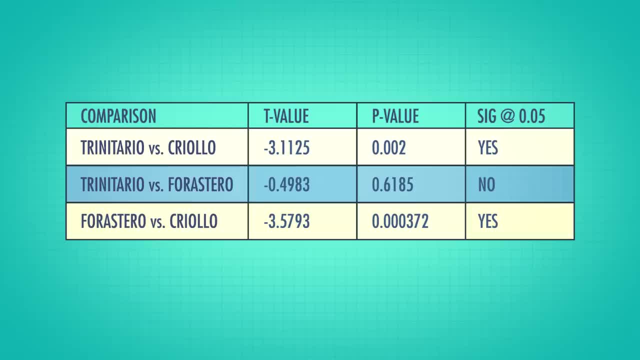 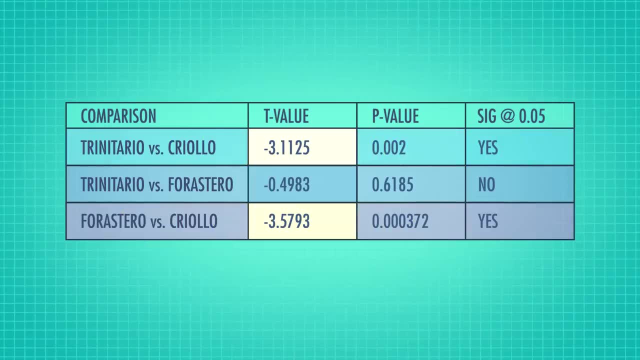 Criollo beans are different in a statistically significant way than those made with Trinitario or F-test, And our graph and group mean show that Criollo bars have a slightly lower mean rating, But bars made with Trinitario beans are not statistically significantly different than. 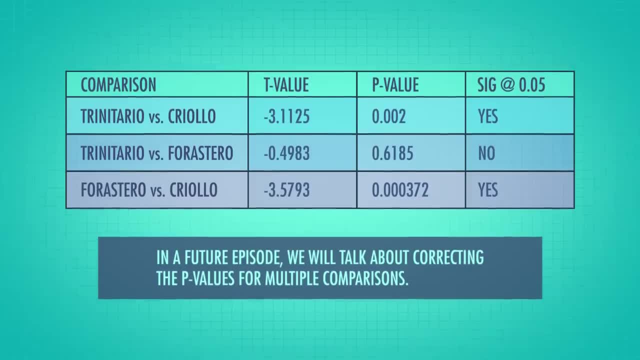 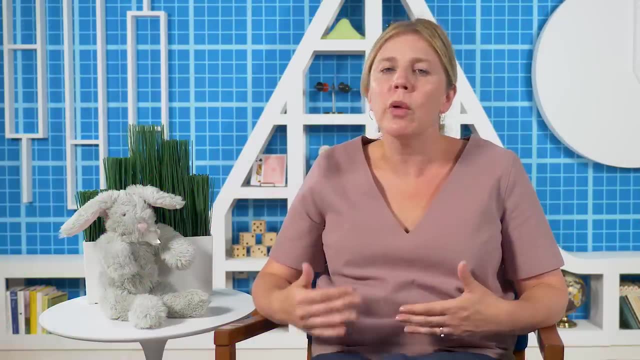 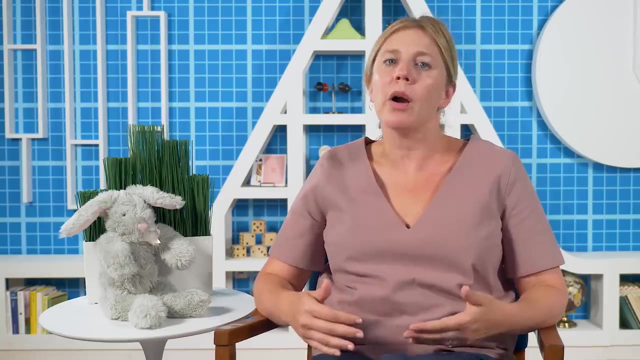 those made with Forastero beans. So our ANOVA F-test told us that there were some differences and our follow-up t-test told us where they were, And this is interesting. Criollo beans are generally considered a delicacy and of much higher quality than Forastero, And Trinitario are a hybrid of the two. 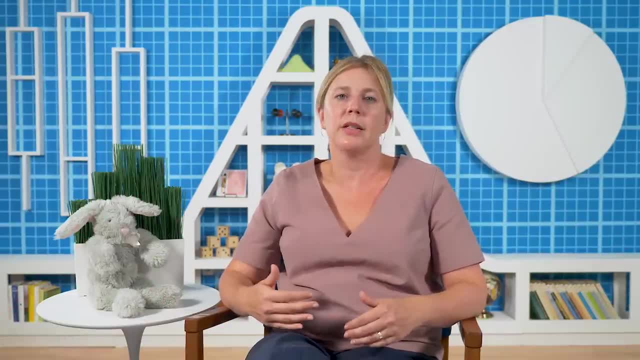 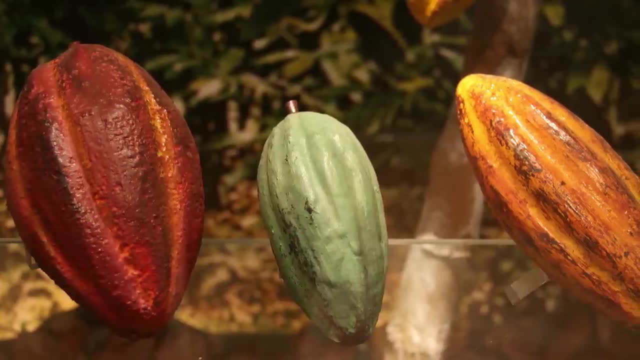 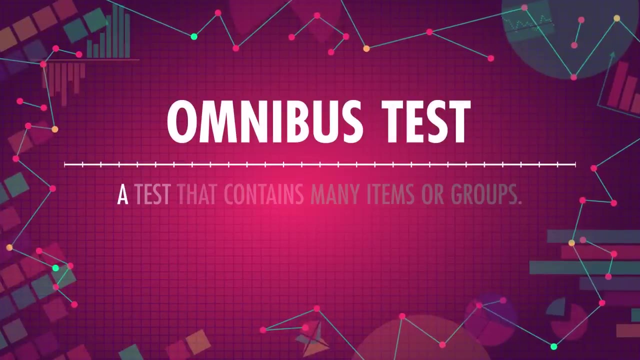 A statistically significant result means that there's some statistically significant difference somewhere in the groups, but it doesn't tell us where that difference is. Maybe Trinitario is significantly different from Criollo, but not for Estero beans. An F-test is an example of an omnibus test, which means it's a test that contains many. 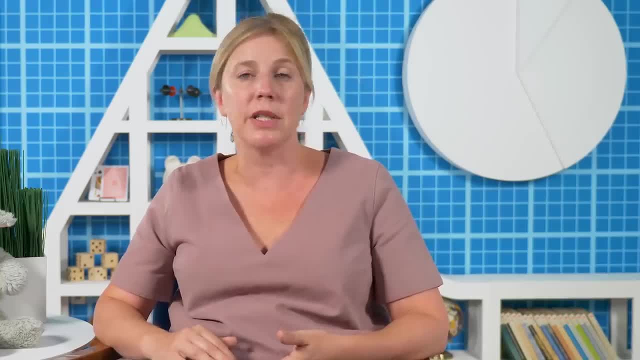 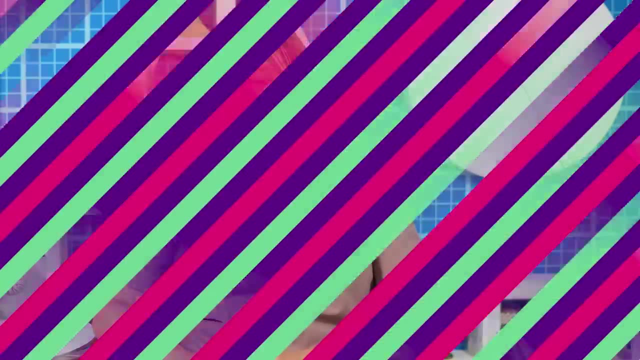 items or groups. When we get a significant F-statistic, it means that there's some statistically significant difference somewhere between the groups, but we still have to look for it. It's kind of like walking into your kitchen and smelling something really stinky. 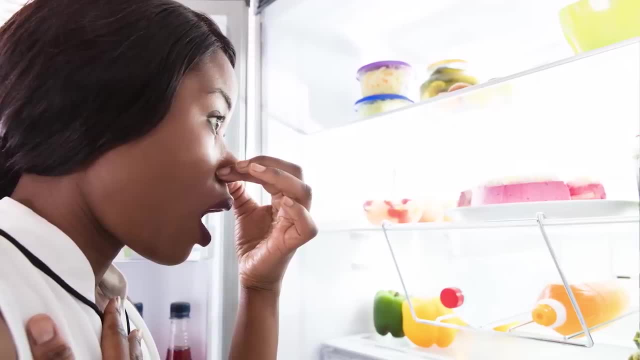 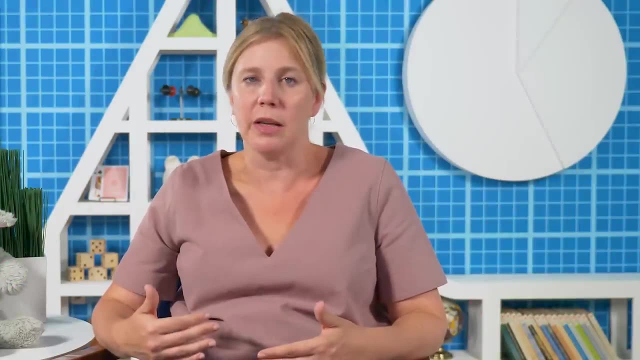 You know there's something gross, but you have to do more work to find out exactly what it is. We already have tools to do this, in statistics at least, because you can follow up a significant F-test in an ANOVA with multiple t-tests, one for every unique pair of categories. your 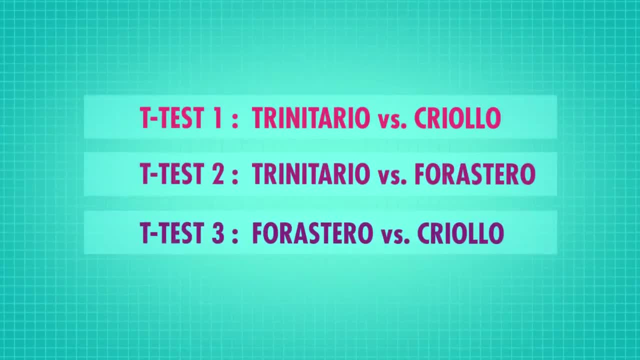 variable had. We had three, which means we only need to do three t-tests in order to find the statistically significant difference or differences. To conduct these t-tests, we just take the data in the two categories for that t-test and calculate the t-statistic and p-value for our final result. 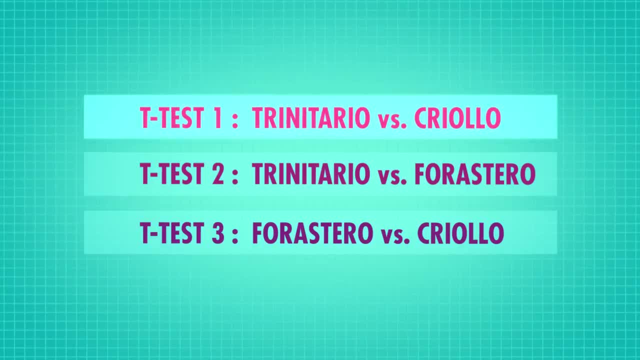 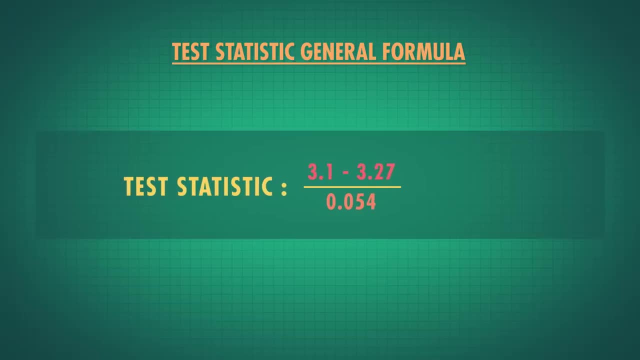 And that's it. Thanks for watching. For our first t-test. we just look at the bars with Trinitario and Criollo beans First. we follow our test statistic general formula. We take the difference between the mean rating of chocolates made with Trinitario and Criollo. 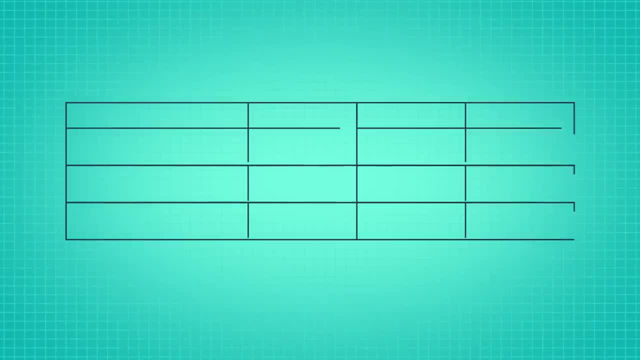 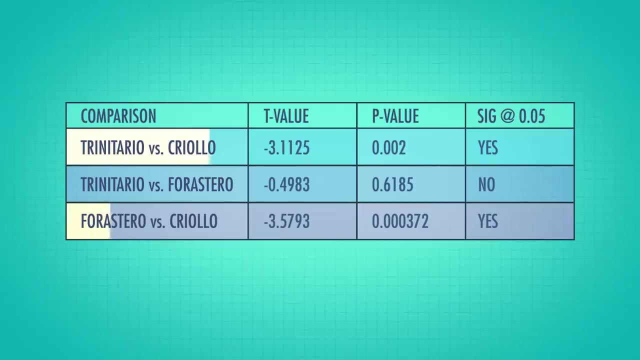 beans and divide by the standard error, And once we do this for all three comparisons, we can see where our statistically significant differences are. It looks from our graph like ratings of chocolate bars made with Criollo beans are different in a statistically significant way than those made with Trinitario or Forastero beans. 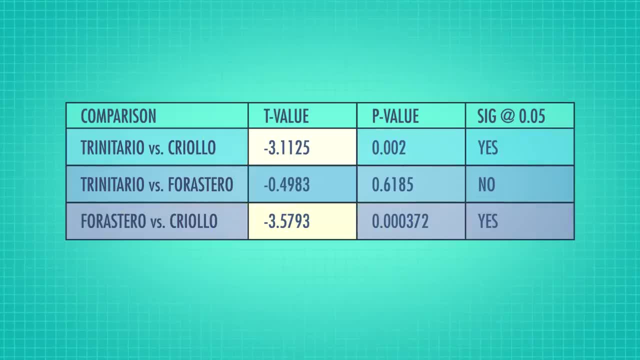 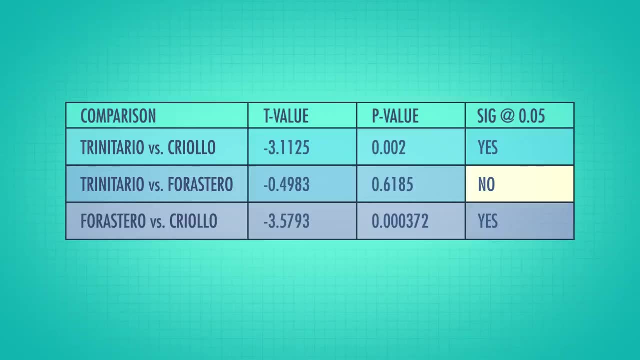 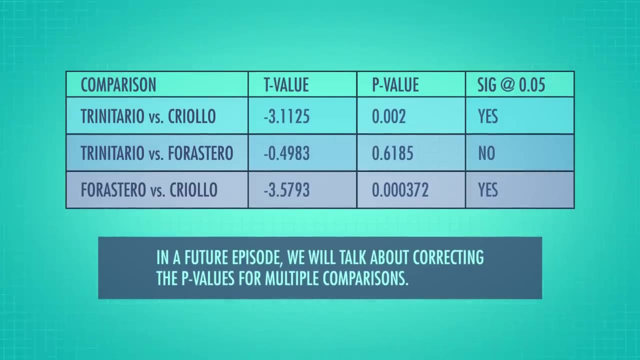 So what's the difference? And our graph and group mean show that Criollo bars have a slightly lower mean rating. But bars made with Trinitario beans are not statistically significantly different than those made with Forastero beans. So our ANOVA-F test told us that there were some differences and our follow-up t-test 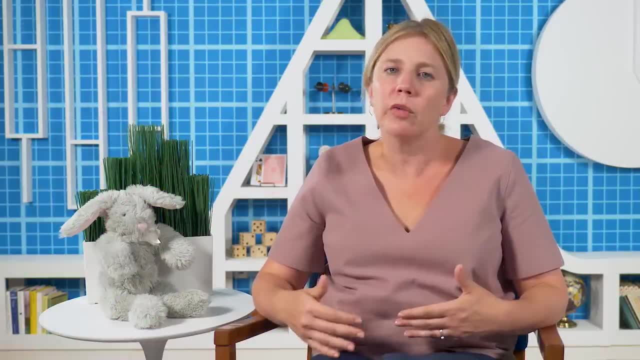 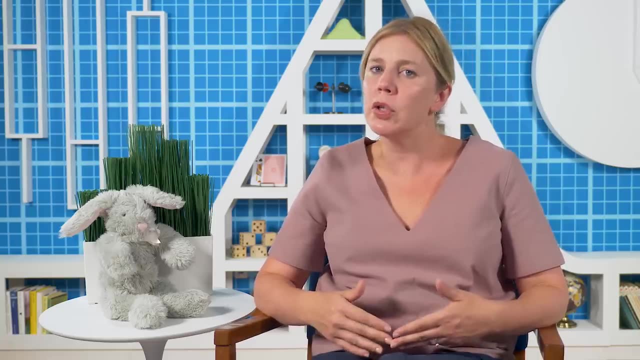 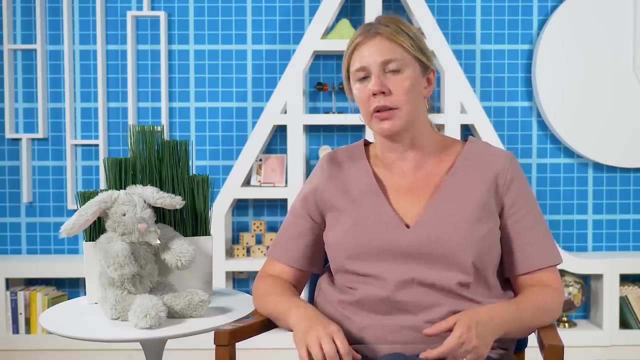 told us where they were, And this is interesting. Criollo beans are generally considered a delicacy and of much higher quality than Forastero And Trinitario are a hybrid of the two, But we found in this dataset that Criollo bars had statistically significantly lower ratings. 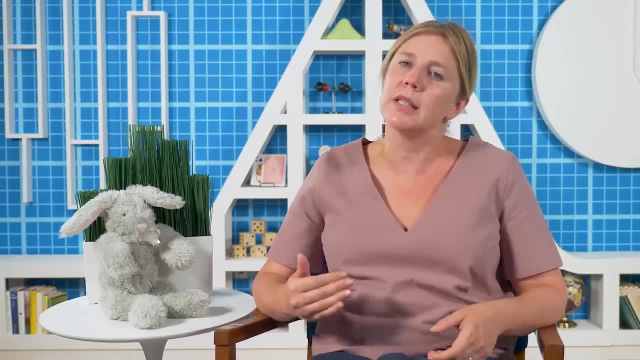 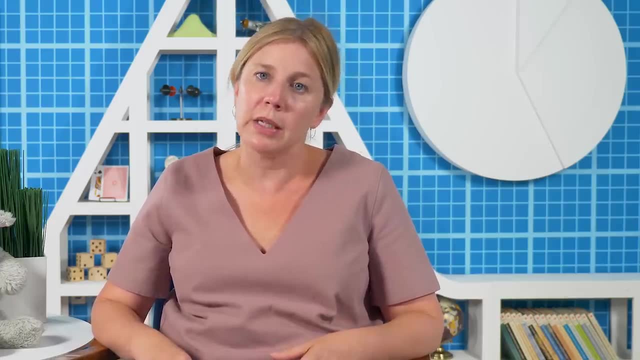 But we found in this graph that Criollo bars have a slightly lower mean rating. We found in this dataset that Criollo bars had statistically significantly lower ratings. This might be because we excluded bars with combinations of our three bean types, or because the rater has a different preference, or even be caused by some other unknown factor. 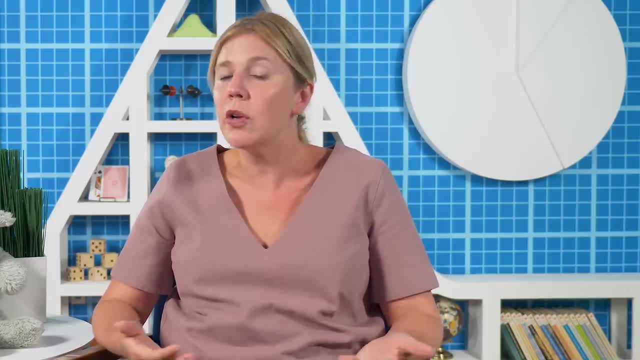 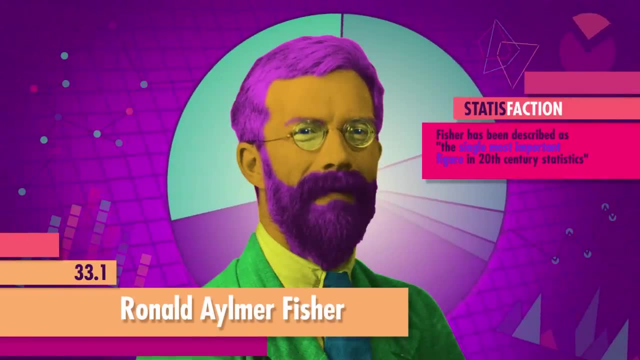 that our model doesn't include, like, who made the chocolate or the country of origin of the beans. We can also use ANOVAs for more than three groups. For example, the ANOVA was first created by the statistician RA Fisher when he was on a potato farm. 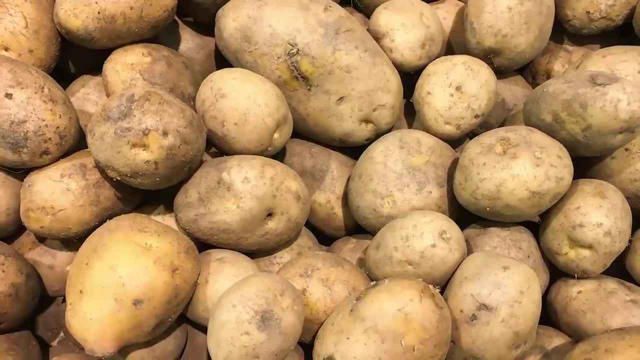 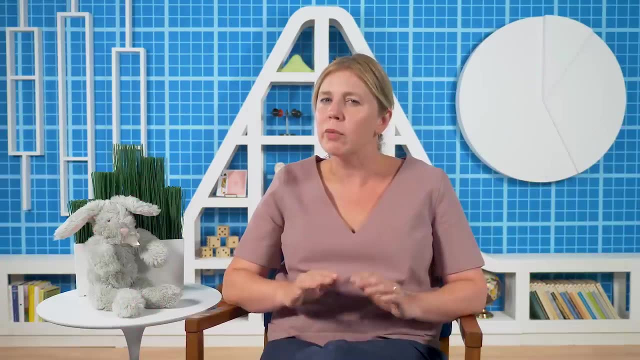 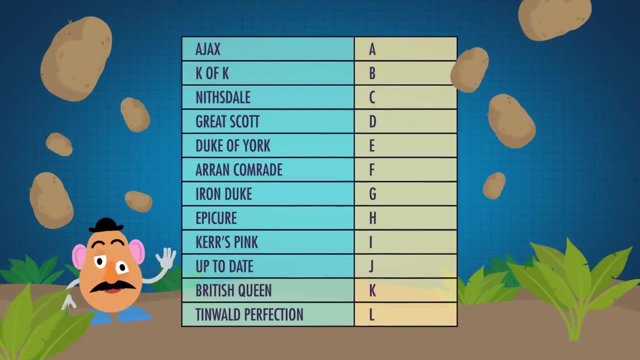 Looking at studies of fertilizer. In one of the first experiments he described, he looked at 12 different species of potato and the effect of various fertilizers. Let's look at a really simple version of Fisher's potato study. Here we have 12 different varieties of potatoes. We'll represent each of them with a letter A. 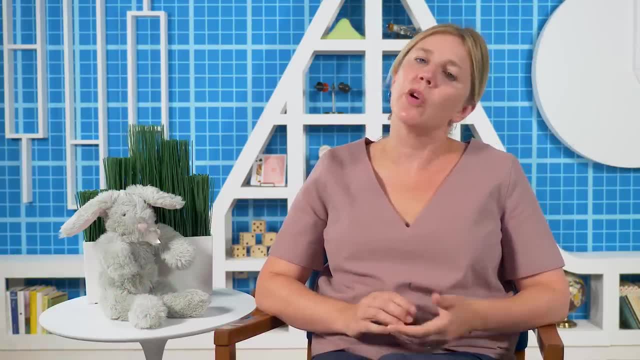 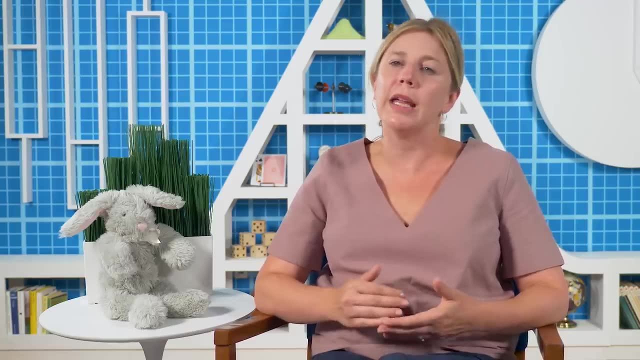 through L. There are 21 of each of the potato plants, for a total of 252 potato plants. We give our future french fries about a season to grow, then dig them up and weigh each one. This shows the potato weights that we recorded, as well as the total mean potato weight. 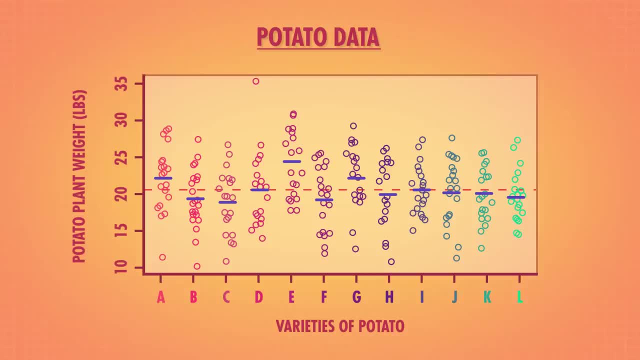 and each group mean potato weight. Using these numbers, we can calculate our total sums of squares. model sums of squares and sums of squares error. We're gonna let a computer do that for us this time, And our computer spit out this: The degrees of freedom. 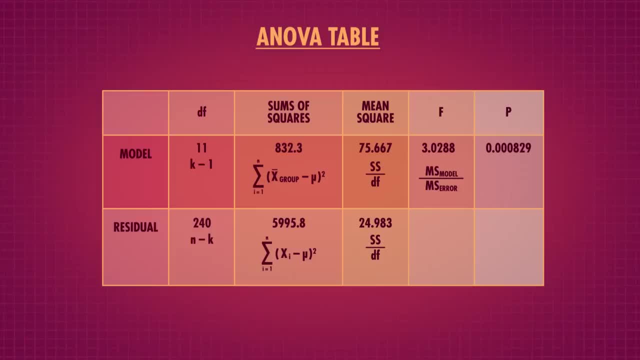 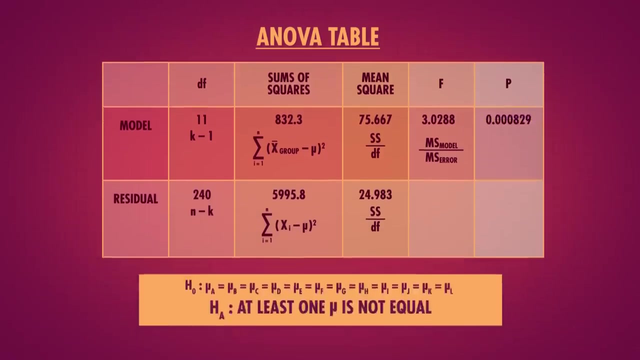 sums of squares mean squares, F-statistic and p-value. This is called an ANOVA table and it organizes all the information our ANOVA models give us. Here we can see that our model has an F-statistic or F-value of around 3, and a p-value of .000829.. So we reject the null. 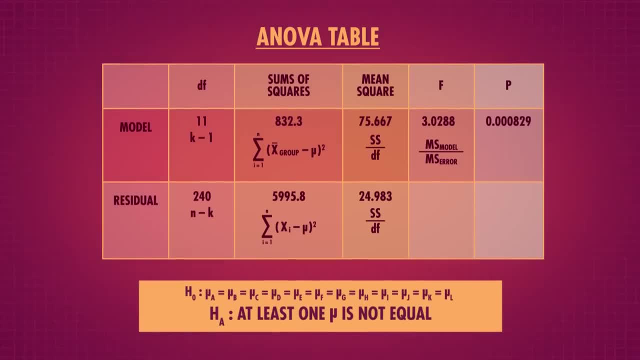 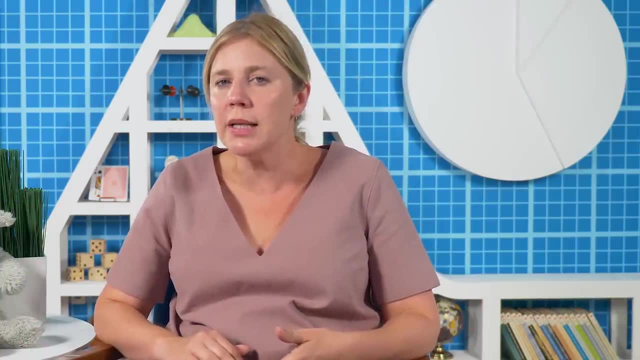 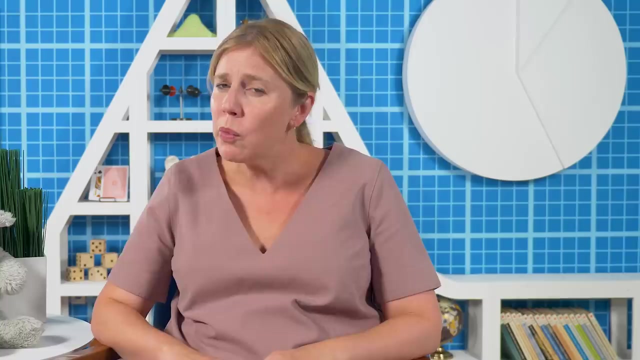 hypothesis, We found evidence that the potato varieties don't all have the same mean weight. But since this was an omnibus test, our statistically significant F-test just means that there is some statistically significant difference somewhere in those 12 potato varieties. We don't know where it is. In that way, ANOVAs can be thought of as a first step. 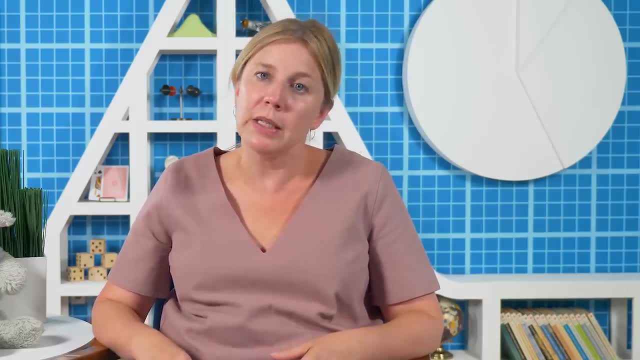 This might be because we excluded bars with combinations of our three bean types, or because the rater has a different preference, or even be caused by some other unknown factor that our model doesn't include, like who made the chocolate or the country of origin of. 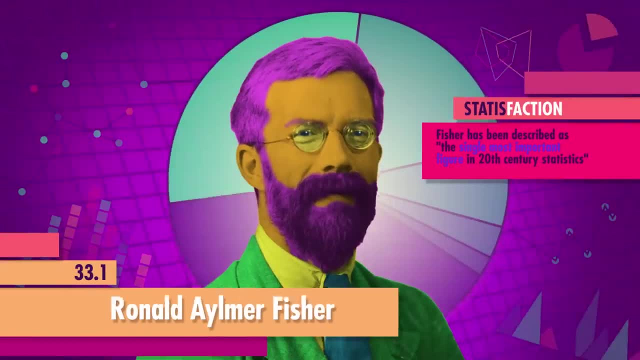 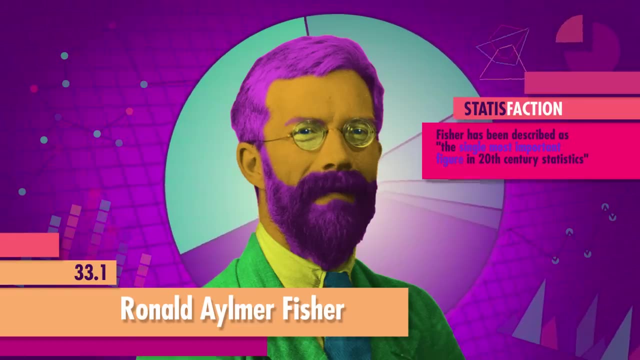 the beans. We can also use ANOVAs for more than three groups. For example, the ANOVA was first created by the statistician RA Fisher when he was on a potato farm looking at studies of fertilizer. In one of the first experiments he described, he looked at 12 different species of potato. 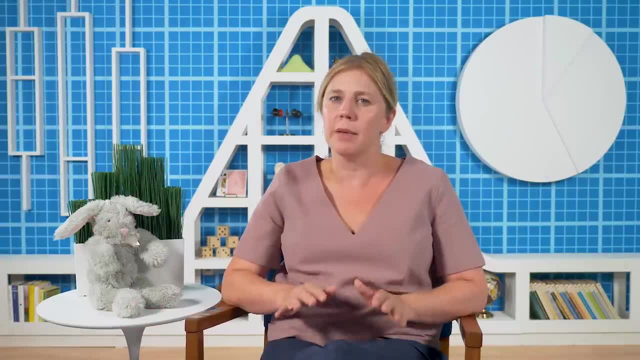 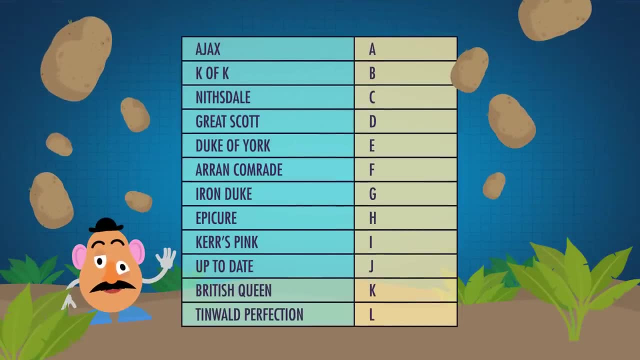 and the effect of various fertilizers. Let's look at a really simple version of Fisher's potato study. Here we have 12 different varieties of potatoes. We'll represent each of them with a letter. A through L, There are 21 of each of the potato plants, for a total of 252 potato plants. 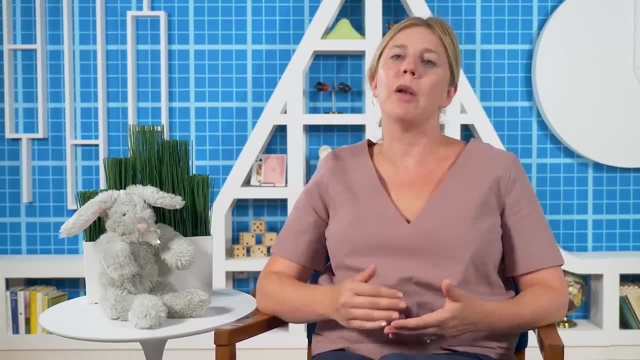 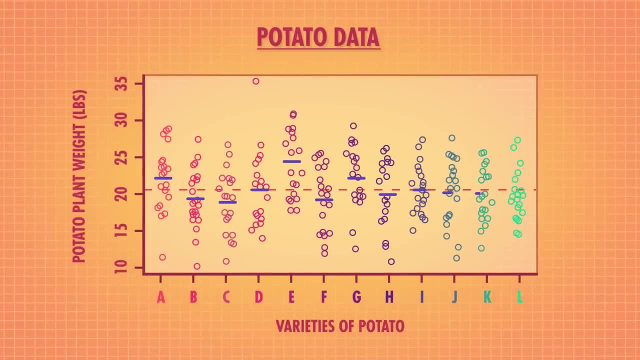 We give our future french fries about a season to grow, then dig them up and weigh each one. This graph shows the potato weights that we recorded, as well as the total mean potato weight and each group mean potato weight. Using these numbers, we can calculate our total sums of squares. model sums of squares. 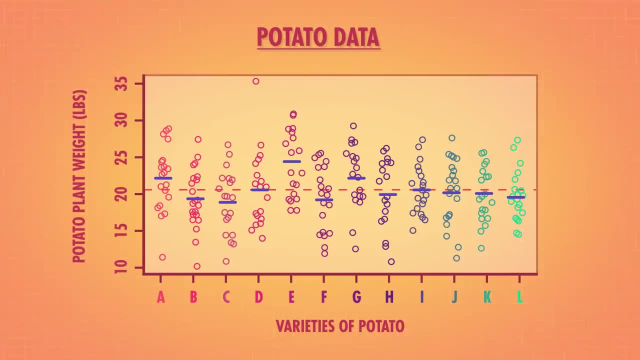 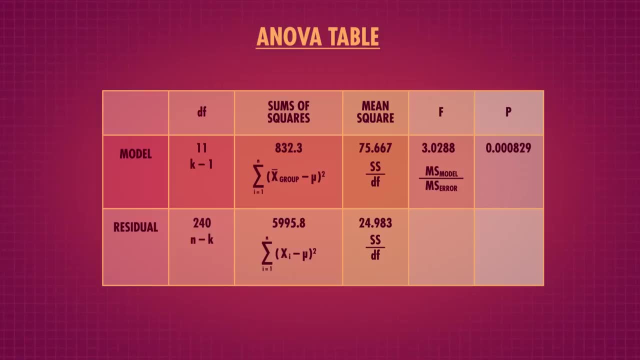 and sums of squares error. We're going to let a computer do that for us this time, And our computer spit out this: The degrees of freedom. sums of squares mean squares f-statistic and p-value. This is called an ANOVA table and it organizes all the information our ANOVA models give us. 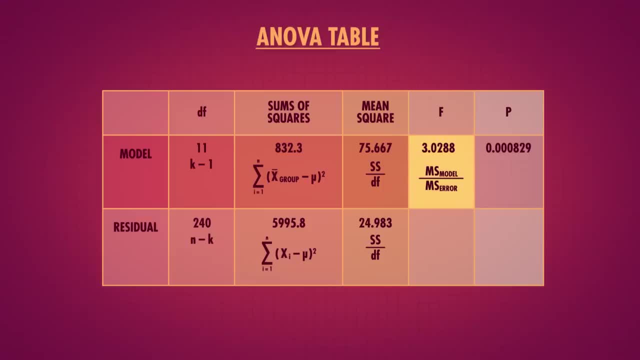 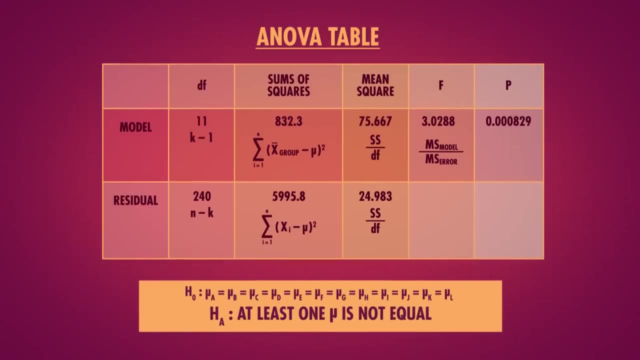 We can see that our model had an f-statistic or f-value of around 3, and a p-value of .000829.. So we reject the null hypothesis. We found evidence that the potato varieties don't all have the same mean weight. 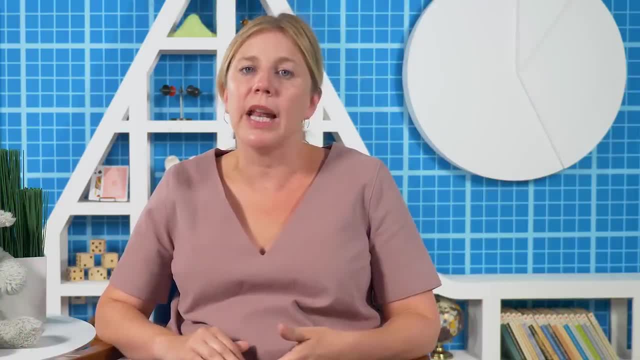 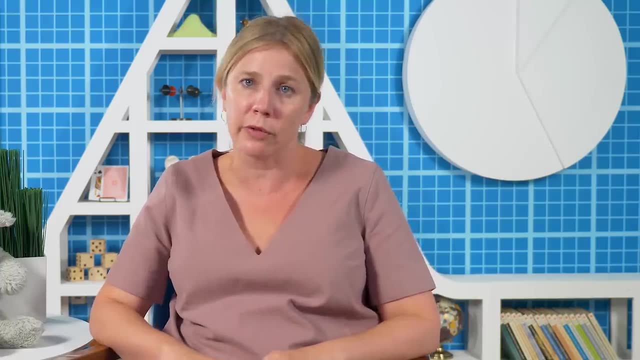 But since this was an omnibus test, our statistically significant f-test just means that there is some statistically significant difference somewhere in those 12 potato varieties. We don't know where it is. In that way, ANOVAs can be thought of as a first step. 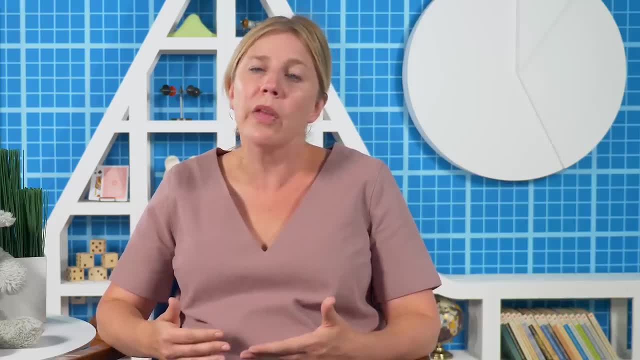 We do an overall test that tells us whether there's a needle in our haystack. If we find out there is a needle, then we go looking for it. However, if our test tells us there's no needle, we're done. No need to look for something that probably doesn't exist.